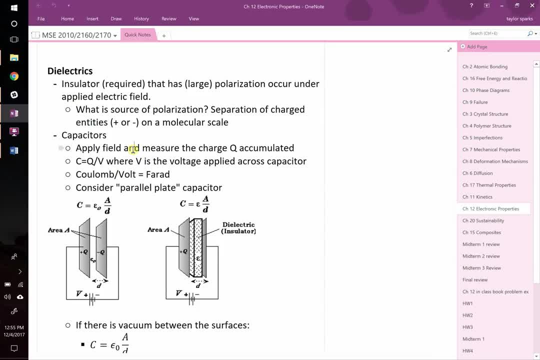 another review for the final exam. in the evenings this week I have to travel for a family thing, So Wednesday will be a formal review. Today we'll actually probably start reviewing, because I just have a little bit left on chapter 12.. A quick note, a couple questions I've had on this. 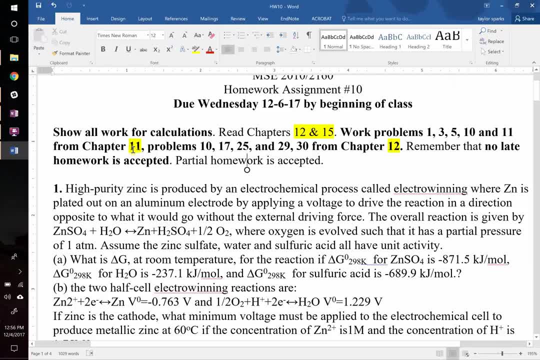 last homework. If you notice, I've asked you to read chapters 12 and 15.. Some years we have enough time to do chapter 15,, which is on composites, as well as chapter 12. here We ran out of time, so that's fine. It won't be on the final exam. You don't have homework questions on chapter. 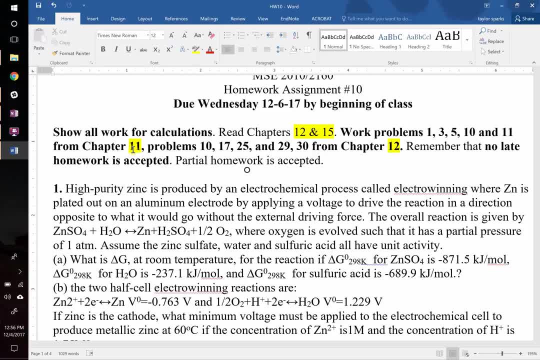 15.. I still think you ought to read it, but it's not something I'm going to be testing you on. So this is correct. I say read 12 and 15, but the homework questions are from 11 and 12.. 11 was kinetics Last week. 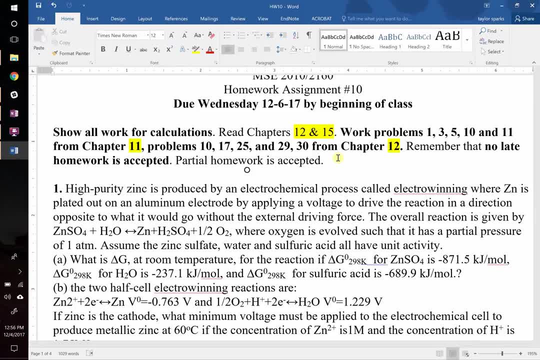 we had the homework. that was the presentation. So I want you to be prepared for the type of questions that we'll ask you on the exam. That's why I've given you some of these, and some of these PDF questions are kinetics related, So that's not a typo. Those are all. 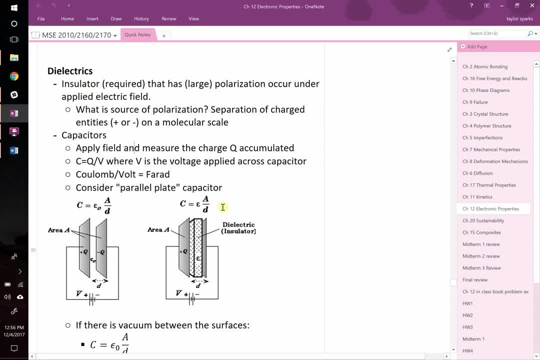 correct. Okay, So today, what we're going to cover? we're going to cover the very last thing. It shouldn't take all the time. We're going to talk about dielectric materials, as they relate to ferroelectrics, piezoelectrics. 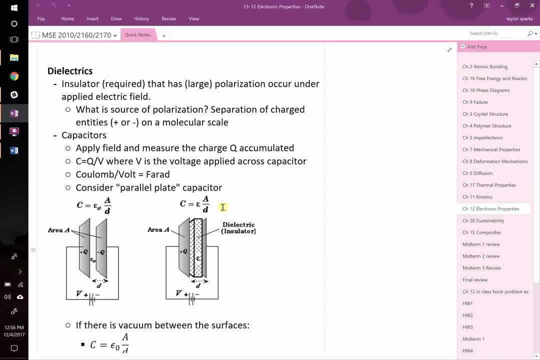 And just a brief thing on some of the devices that we can make out of those materials once we have them. So what exactly is a dielectric? Why do we care about them? What do they do We care about them? if you go back to what we were talking about last class, when we talked about the 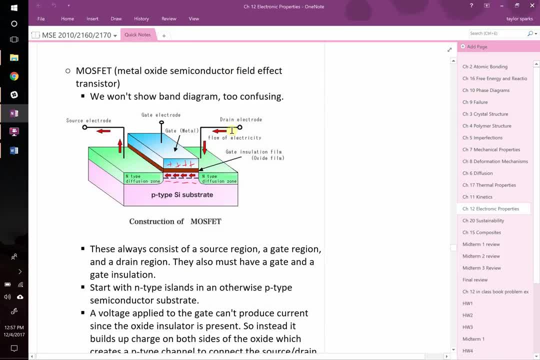 MOSFET. So right here the MOSFET. if you remember what the MOSFET was, that stood for metal oxide, semiconductor, field effect transistor, right? So the dielectric comes into play in this example, in this little brown layer as it's drawn here. That's the oxide. Now, that material does not. 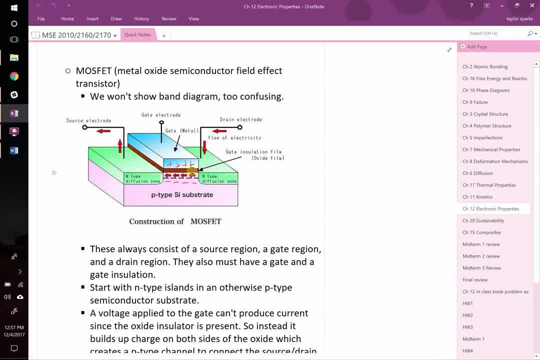 conduct electricity. It's got a great big band gap right That material, But what it does do is that if you apply a voltage to it right, you can make it a gate. So what they do is they apply a voltage to it- In this case they apply a positive voltage to it right- And what that does is you. 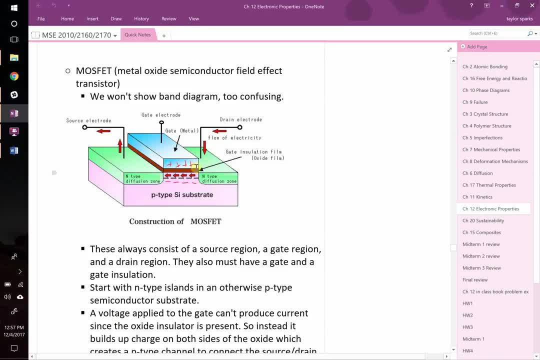 get this accumulation of positive charge here in the metal layer, right at the surface of the metal, in the oxide, And to have charge balance out. if you accumulate positive there, you have to accumulate negative on this other side And that's what makes this channel actually exist. So these 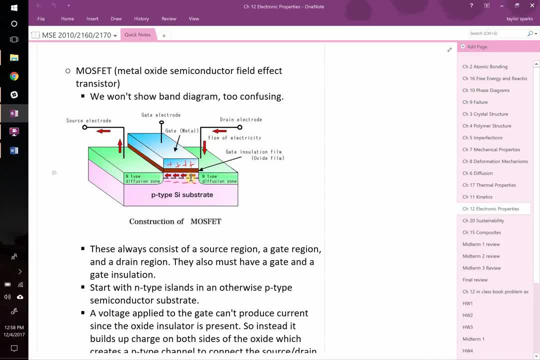 type of semiconductor transistors. they only work because that oxide material has a high dielectric constant, which is something we're going to talk about next. Yeah, Arthur, So good question. The substrate, the silicon, the silicon and the silicon. they don't really do anything to it. It started out as p-type. 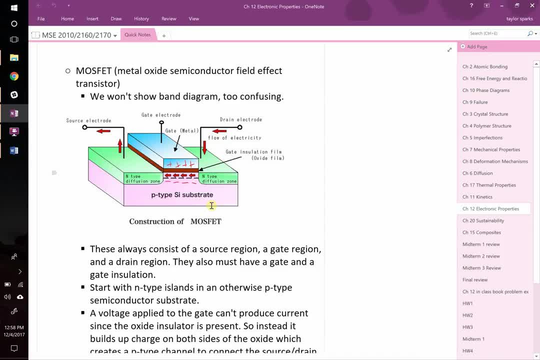 The first thing they did, is they probably via ion implantation, but they might have done photolithography and masked in diffusion. right, But some way or another they introduced. what Did they introduce? acceptors or donors into these green regions? Well, the bulk is p-type. P-type has holes. These are now N-type. What do we do if we want to make? 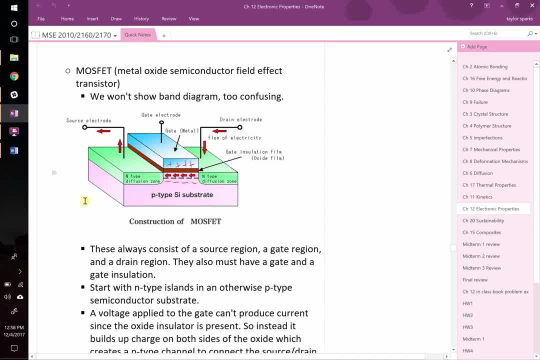 something N-type, We want to give it holes, or electrons. Electrons, So we're going to give it donors or acceptors. Donors, Donor, right. so if this is silicon, you might have put something like phosphorus here. so they either ion implantation. 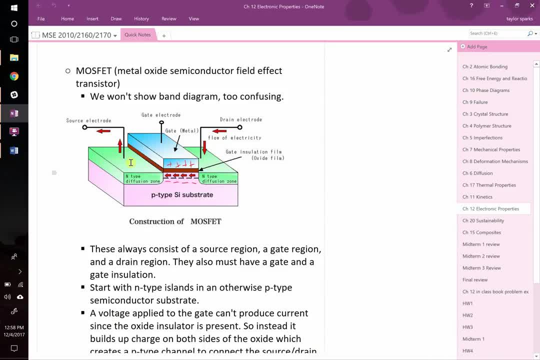 They painted this thing with phosphorus. however, They did it. they put some phosphorus on there right. then they heat it up and let that phosphorus to fuse in, and now you've Got some region which is now n-type. you've basically given it lots of electrons. 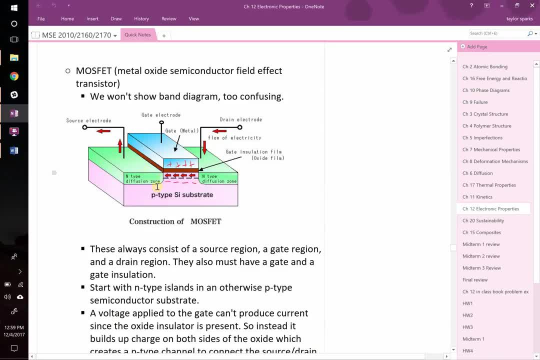 So if you did nothing else, then you'd have two pn junctions. You'd have a pn junction, one right here, and on the right hand side you'd have another pn junction. But the way that this works as a transistor is really clever. We won't get into the details of it in this class. 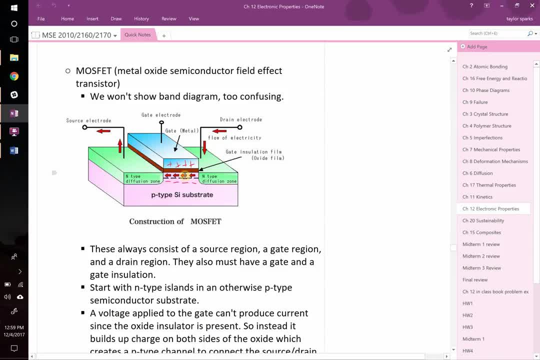 But it suffices to say that if you induce the, the existence of these negative charge where these little arrows are, That's kind of the same as putting electrons there right. negative charge, those are electrons right. so what it does is it creates a pathway. You knew the electrons conducted in the green region and all of a sudden, 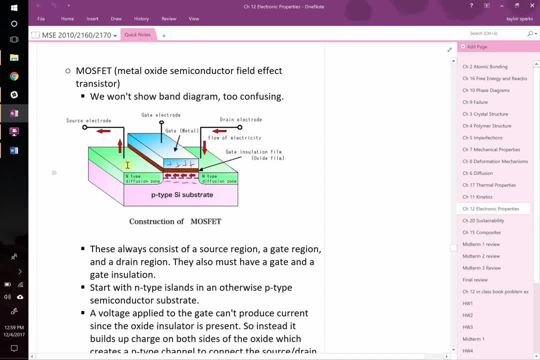 You've got a little pathway where electrons can conduct to this green region. So you've got a transistor, you've got, when that voltage is applied and those negatives are there, you have a pathway. When that voltage is not there, you don't have a Pathway. recombination would occur. you basically have an LED, but no current would get through. that makes sense. so yeah, you do have two pn. 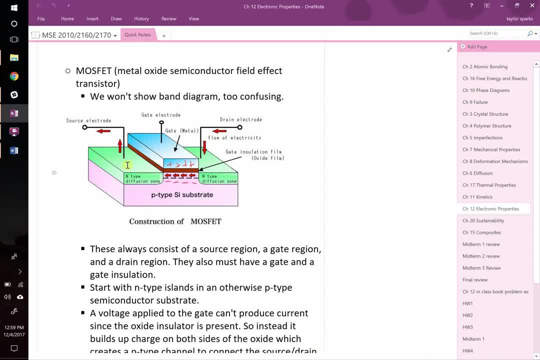 junctions. But you have something special that can happen: you've got two pn junctions. that turns into just a regular n Channel when you apply that voltage. and that voltage only works because you have a dielectric which allows you to accumulate charge on the surfaces. Yeah, Rosa. 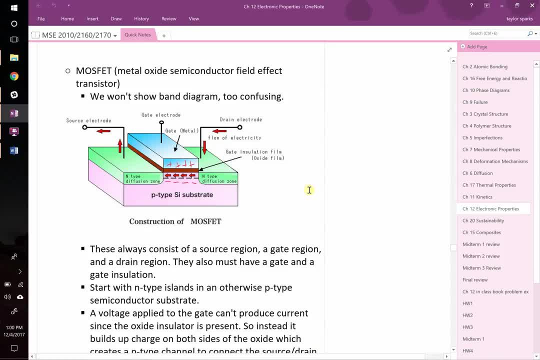 When did you put a donor on that? Okay, Okay, How do they? Is that like just a whole Green part of it? Will that? Is it like unequally diffused? It's a good question, So I'll say it's very, very difficult to get like. if you were gonna like 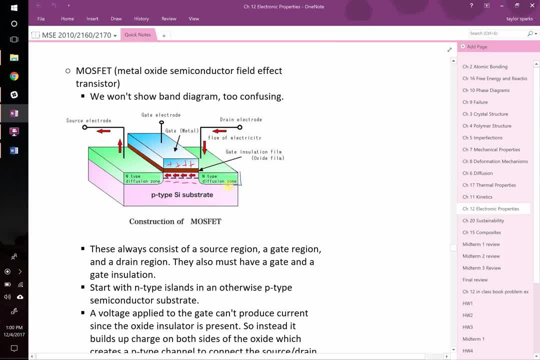 Try and create exactly like it's drawn here, Where there's like n-type and a specific depth. where there isn't, that's gonna be really hard to achieve, Because what do we know about diffusion? We know about diffusion that if this is X going into your material and you have some initial concentration here at the surface, 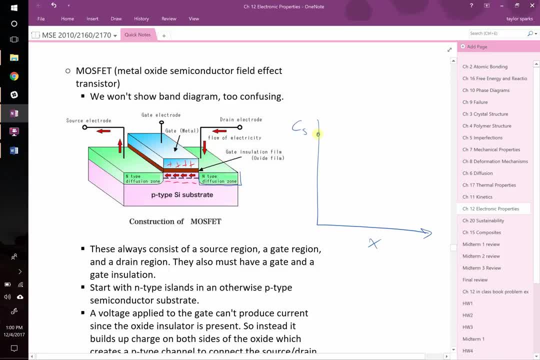 We know from fixed-second law, which we've seen over and over now, that it starts to do this thing at a short diffusion time. It does that. if you let it hold longer and longer and longer, it starts to do that. at no point, though, Does it go like that right. 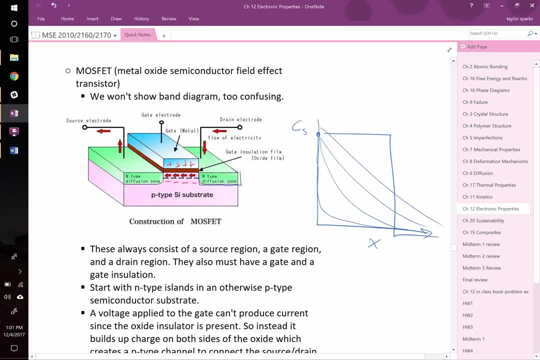 So you're not going to be able to achieve that using diffusion. you can achieve something kind of like that with ion implantation. ion implantation when you take something like your phosphorus source and you come up with a way to Accelerate it and crash it into your silicon, because then they might all sort of crash at a similar depth. 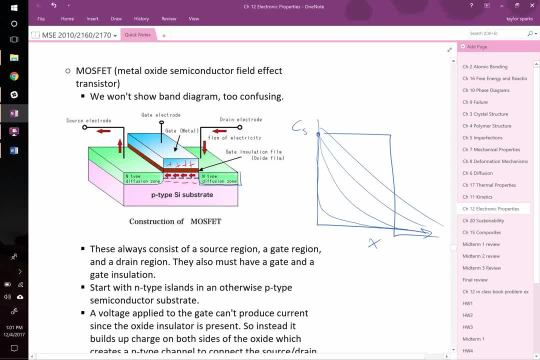 So you might be able to achieve a profile like that, And I'm sure that clever engineers have come up with other ways that I'm just not thinking of right now. But yeah, those are the tools that they typically use. Other questions on this. Again, the whole reason I bring this up is this thing that we sort of took for granted. 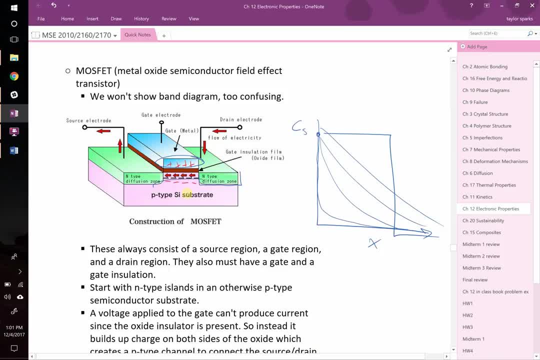 We said, okay, you apply a voltage to this, you accumulate positive charge, You accumulate negative charge, But we haven't yet described why that even happens. Why do you accumulate charge on the surface of something? right? So to describe that, let's move down and talk about dielectrics a little bit. 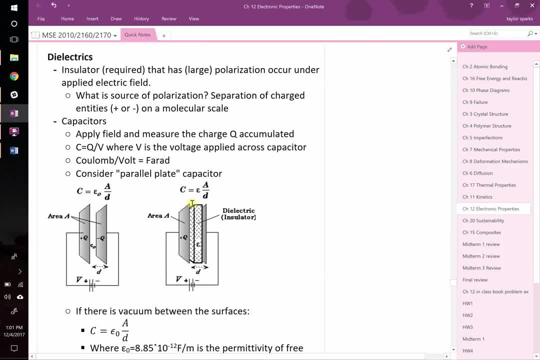 So dielectrics: right, They create a polarization, an electric polarization Under an applied electric field, right. So normally, if I took, if this was my piece of, say, a metal And I hook a battery up to it on either end, I've now applied an electric field across this thing. 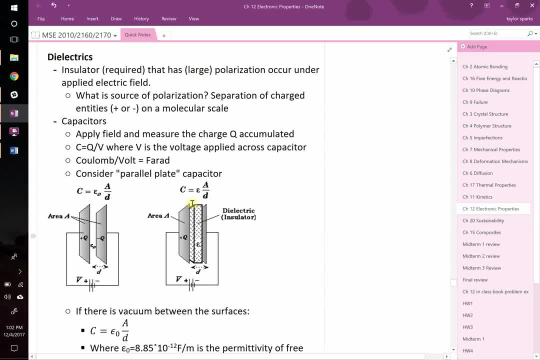 But I don't create a polarization where, Where I accumulate charge on the surface On the two sides, that doesn't do anything. Instead, I cause electrons to travel in this thing Because it's a conductor. if this was a piece of metal, right, But imagine if this thing doesn't conduct electricity. 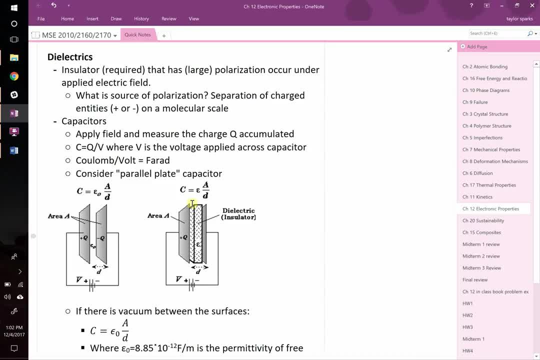 And I hook up a battery to it. Now, since electrons can't travel through it, All I can do is I can store them on the surfaces where I attach it right. So because of that, they call these capacitors, And specifically they call them parallel plate capacitors. 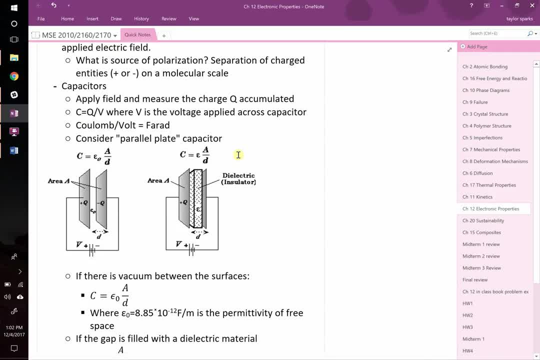 In physics you've probably seen something like these already: A parallel plate capacitor. Here you've got your battery with some voltage. You're going to hook the positive and the negative ends up To two pieces of metal that are parallel but not touching. If those were to touch then you'd just have a circuit. 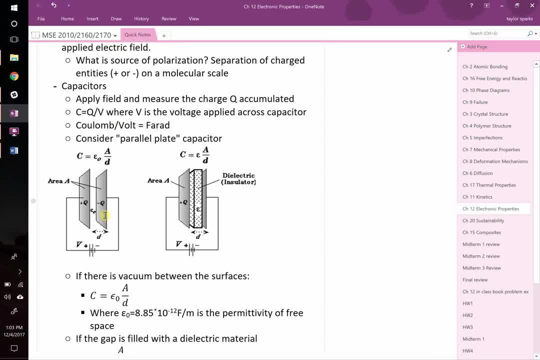 You'd have a current running through it. Whatever the resistance of those metal is Would dictate how much current for a given voltage. That's not interesting. What's interesting is if you have them not touching, Because now if you apply a voltage, You can't have a current running through this thing. 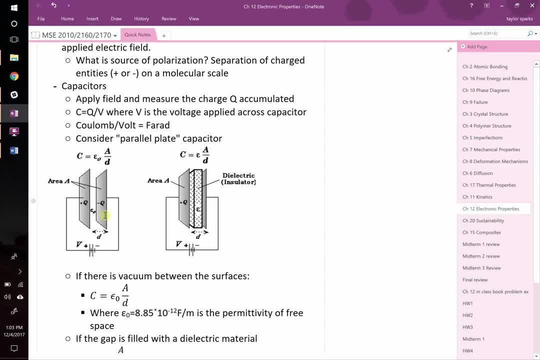 So what can you do? Well, what you can do is you can shuttle electrons. Let's say, we shuttle some electrons over to here And they just sort of pile up on the surface of this thing, And in doing so that's going to induce a positive charge. 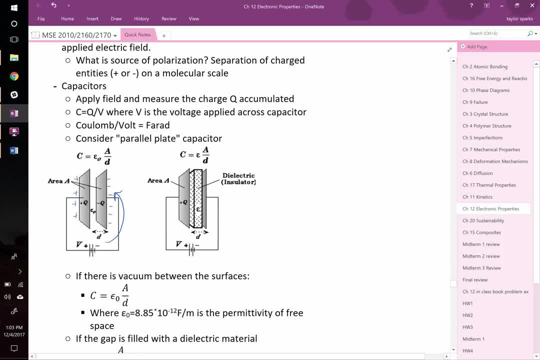 Basically, those electrons had to come somewhere in the wire. So from the wire they're traveling from this region over to that region, Accumulating negative, accumulating positive Right. And if you have this hypothetical metal which is just this perfect conductor, Then you can have a parallel plate capacitor with nothing in between. 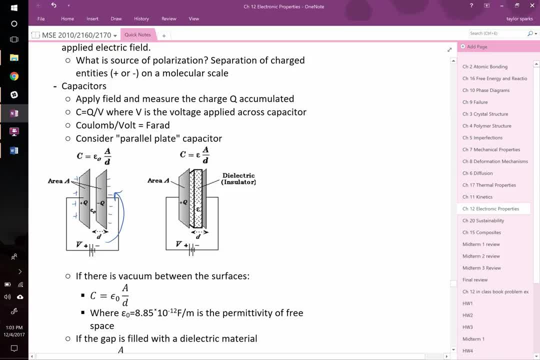 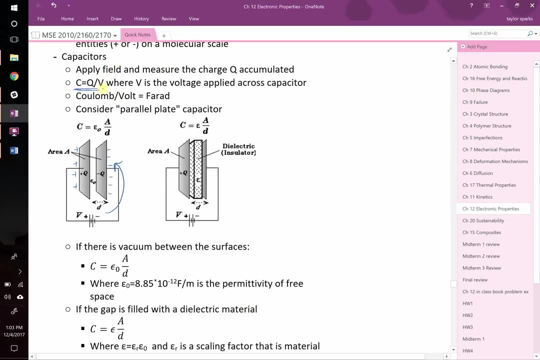 Right, With vacuum in between, if you want to call it that. And if that's the case, We can calculate what will be our capacitance. What is capacitance? Capacitance, by the way, is just equal to charge Q For a given voltage, Right? 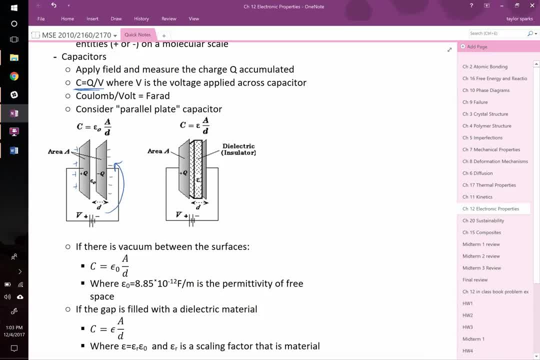 So if you apply 9 volts Right And you accumulate X number of charge in coulombs, You could calculate the capacitance Right. Take that charge, divide it by the voltage, You got your capacitance. So the capacitance of this perfect parallel plate capacitor. 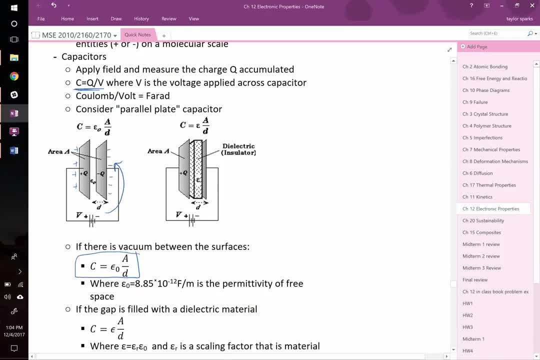 With nothing in between. Just the vacuum Is given as epsilon naught. Epsilon naught is our permittivity of free space. It's a constant. You learned it in physics, It's given right here. That's going to be multiplied by the area of your parallel plates. 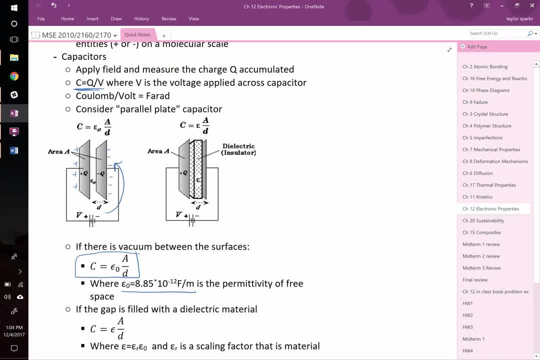 And divided by the thickness Right. So if you want to store more and more charge on something, Let's say you want to create a super capacitor. If you've heard of these, You guys heard of super capacitors, right, They're basically in competition with batteries. 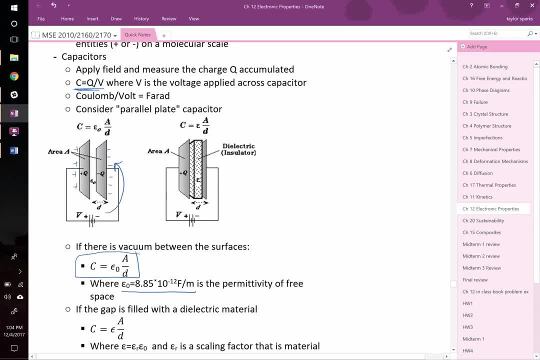 Like, how could you store charge in something? Well, rather than electrochemically, which we've done all semester, You could just store charge on surfaces When you want to use it. You short these things out And allow that charge to go somewhere right. So if you're going to store a lot of charge, 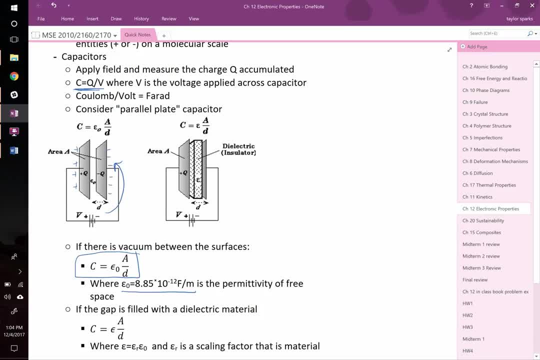 You'd do one of two things: You'd either take a really big surface area, Make A as large as possible, Or you'd bring these plates as close as you can together, Because either of those things Will let you store more charge for a given voltage. Any questions so far? 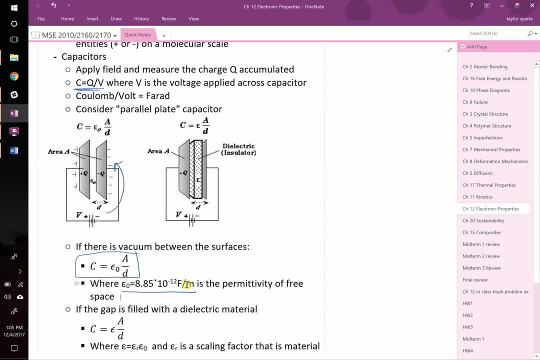 Okay, that's a parallel plate capacitor In the real world when we make- Yeah, Arthur, So you were talking about super capacitors- Do the people that make those? Do they prefer having a smaller distance or a bigger area? They do bigger area, And the reason why is because 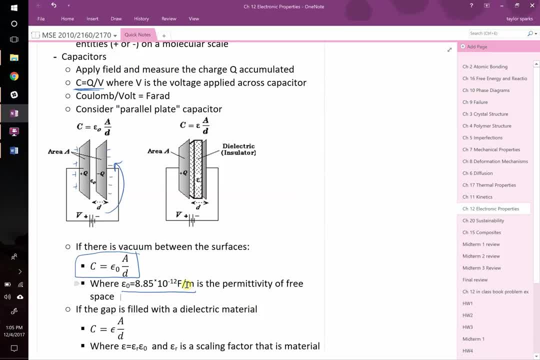 There comes a point when you're bringing these really close together That it's really hard to avoid them shorting out and touching Right, Because if they touch Even in one spot, that could ruin your whole capacitor. All your charge is just going to cancel. The positives will meet the negatives. 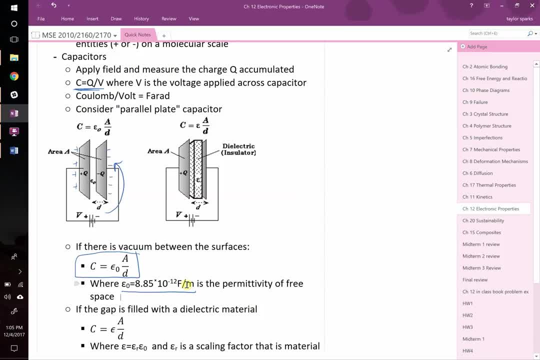 You'll generate a bunch of heat and you're done Right. So it's safer to set some minimum controllable thickness And then try and grow your surface area Like crazy. So that's what they do. They make actually not crazy thin things, But they try and get really high surface area materials. 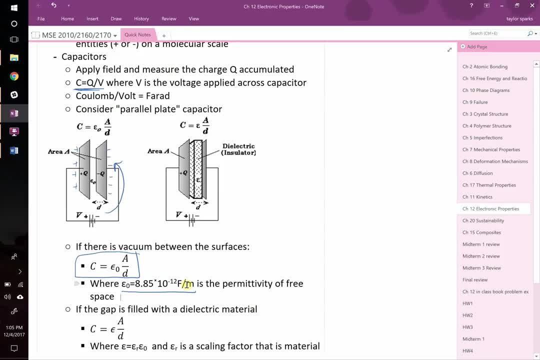 Like tiny carbon, right, You take carbon black that has a pretty high surface area And then say: what about carbon nanotubes? right, You can store the charge on either side of these carbon nanotubes, And they come up with all sorts of games like that. 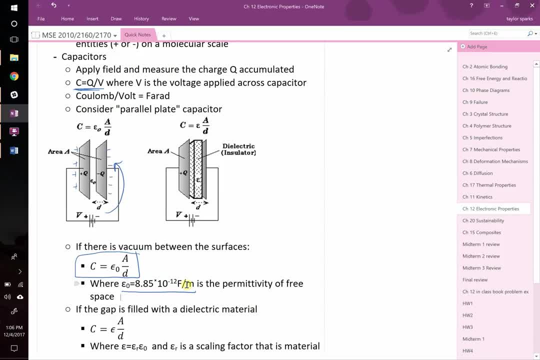 And they're getting pretty good. The total amount of energy you can store on them Is not anywhere compared to batteries, But the power, Which is the rate that that energy can be delivered, Far exceeds batteries, Right. So capacitors are great for high voltage, low energy applications. 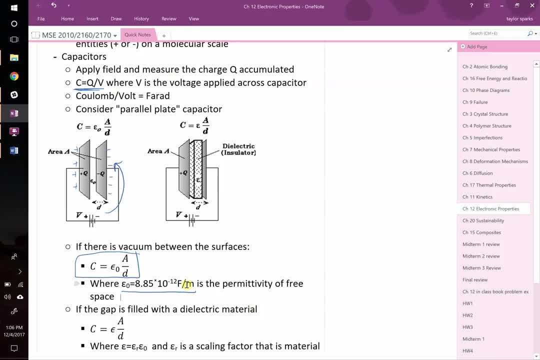 And batteries are better for the opposite. Right, And lots of hot air research in that area. I just don't work on it myself. Okay, You can do it with vacuum, right, Pull this thing out of vacuum, Bring these plates close together. But that's not what they typically do. 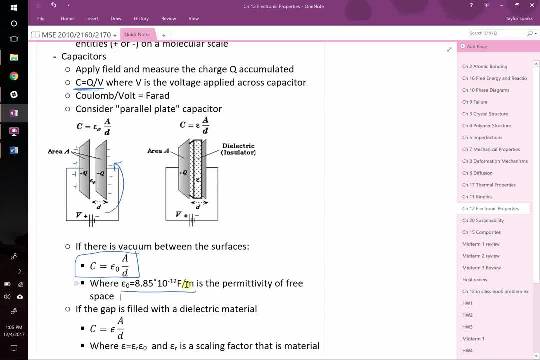 Because you can get a multiplying factor If you put something in between there, As long as, whatever it is you put in between, there Is a dielectric material, Meaning it's not going to conduct electricity And it's going to help you accumulate charge, Right? So this insulating material, 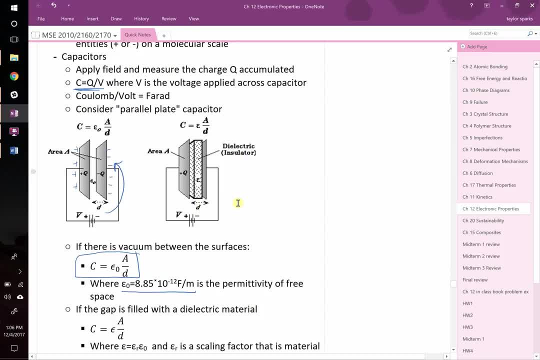 Which they're showing in this sort of cross hatched area. You put that inside of there. When you put that inside of there, The total capacitance you can achieve Is now no longer epsilon naught Like in the vacuum case. It's now what we just call epsilon. 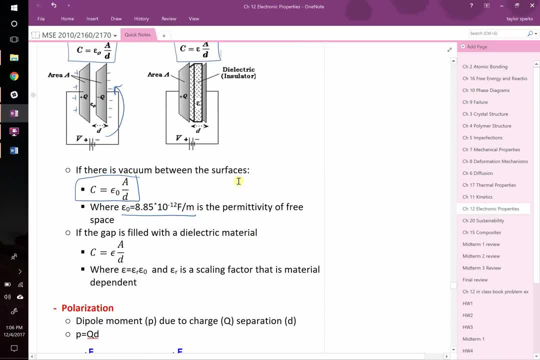 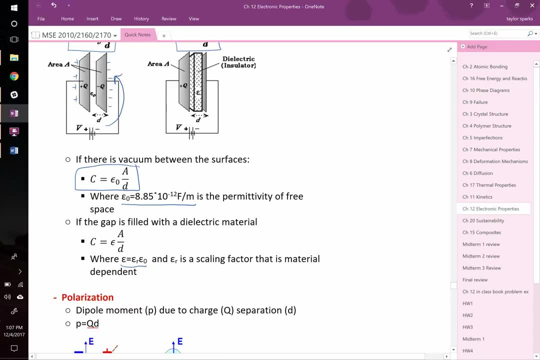 And epsilon itself is equal to Right. here It's equal to epsilon naught multiplied by epsilon r. Just some factor, It's a constant Right, It's a number. So by putting anything in there You get a better dielectric Or a better capacitor than vacuum. So vacuum is the worst case scenario. 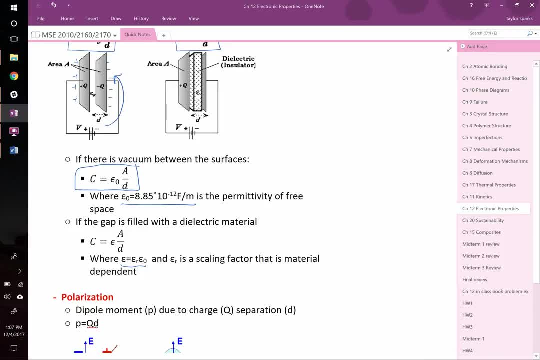 Put anything in there As long as it doesn't conduct electricity- And you made a better dielectric. You can hold it more. So what are those numbers? I think we're going to talk about them in a minute, But typical values can be quite low For a long time. 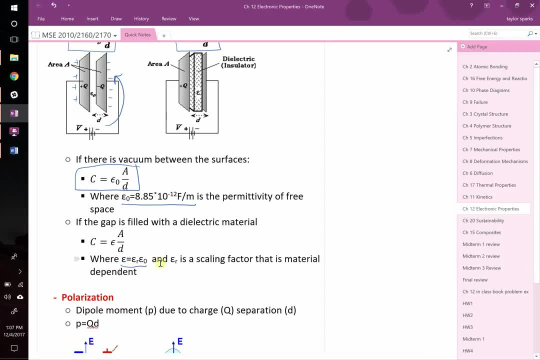 The best things they had. They would use clay and mica. Water is actually not terrible: Pure water that doesn't conduct electricity, And they're like less than 100, I think, Or right around there, So you can get maybe 100 times better than vacuum. Nowadays we have things. 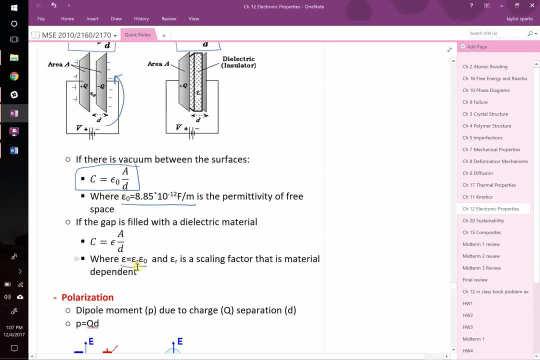 Where this dielectric constant E sub r Can be thousands Right Or tens of thousands, even Just monstrously high, And we'll talk about why that is in a second. Any questions so far on capacitors? Parallel plate capacitors: Yeah, Anders, To my knowledge no. 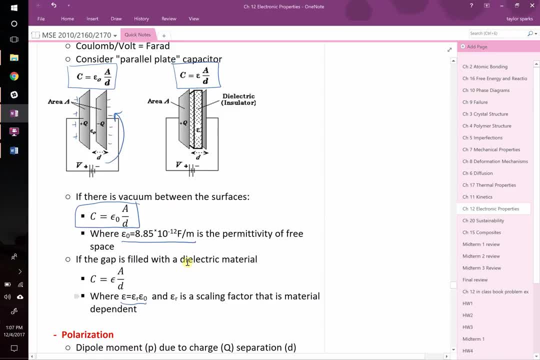 I don't think so Because, again, Vacuum is sort of not better Than anything else. Right, You can make something better By adding a dielectric constant there. And vacuum is sort of better Than anything else. Right, You can make something better By adding a dielectric constant. 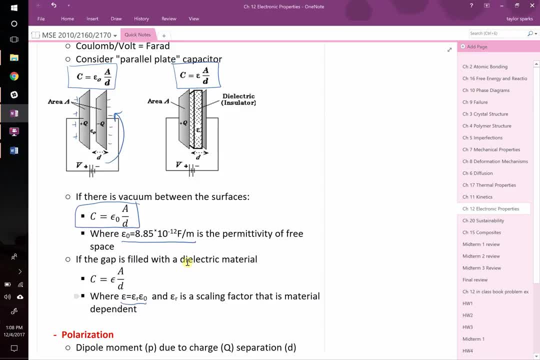 There, And vacuum is sort of better Than anything else, Right, You can make something better By adding a dielectric constant there, And vacuum is harder to work with And more expensive And it fails, Right? So I, To my knowledge, They don't do anything And I can't think of a reason why. 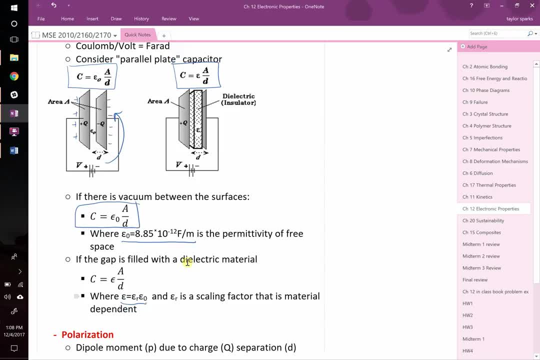 But there could be Other questions. Rosa, No Great question, though. In that material You've got Two plates, Two ceramic plates, And those are separated By a series of P And N type Semiconductors Right, So the electrical current Passes through those. In this sort of 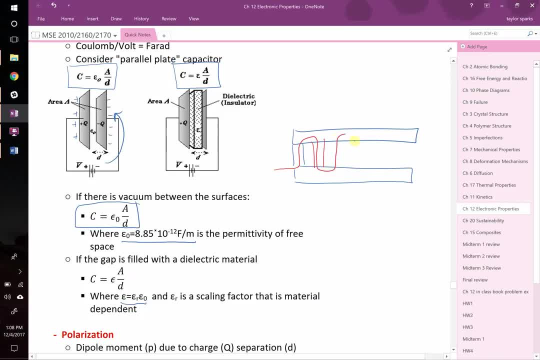 Snake-like Semiconductor, Semiconductor Right Snake-like pattern. So they're connected In what we call Series electrically But they're thermally In parallel, So heat travels Just through it All in parallel, But the electricity Has to travel Through those In series, So this Conducts electricity. 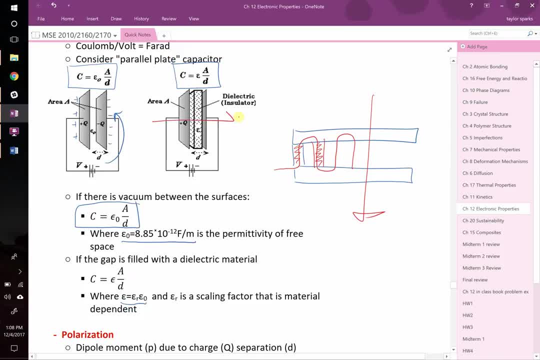 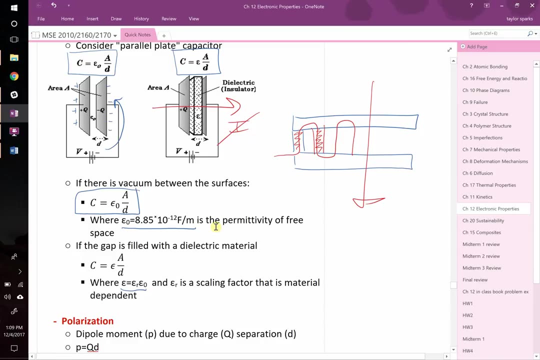 Throughout. What we're talking about here Would not conduct electricity. There's no current That goes Across that, Right, No current is allowed, Right. Other questions I can answer: Okay, Let's keep going, So, Alright. So we have A material, This dielectric, That just We put it in. 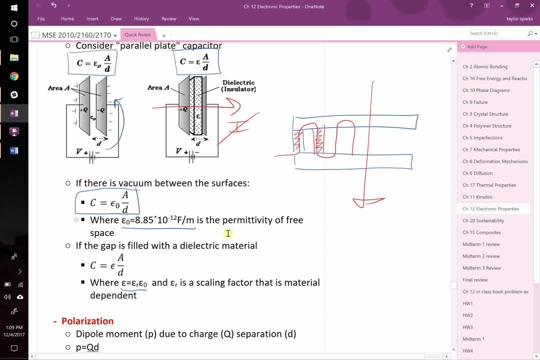 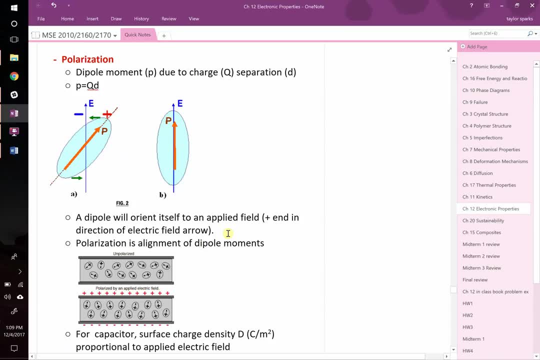 And it makes our capacitors Way better, A hundred times better, A thousand times better, Ten thousand times better, Right? So what on earth Is going on To explain that We have to introduce The concept of polarization And where polarization Comes from, In materials. So a polarization. 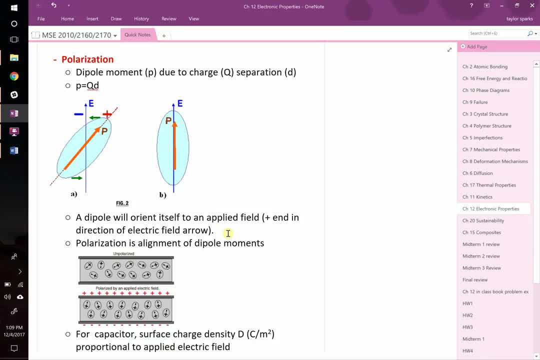 You would have seen this In general chemistry. In physics, Polarization is just A dipole moment. Right, And a dipole moment Is equal to A charge molecule for a minute. right Water molecule, it's H2O. right, So you've got your oxygen. 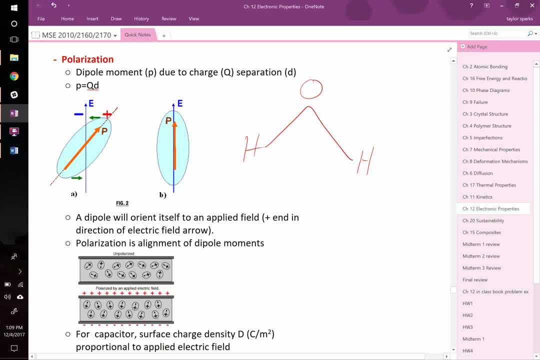 and you've got your two hydrogens. We know it's a bent molecule. The reason why is because oxygen has these two lone pairs right, So that leads you some angle that's kind of like 109.5.. It's actually squished a little bit right, So you get this bent molecule right. 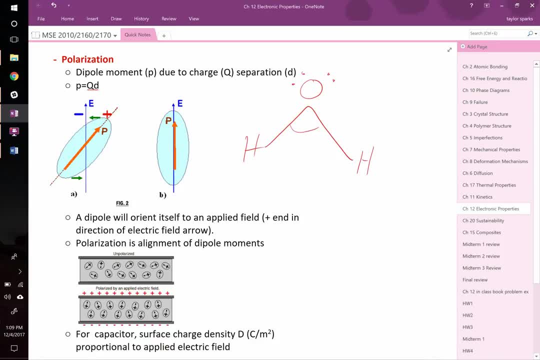 That's water. Now, what wants electrons more? the oxygen or the hydrogen Oxygen definitely does. So it's going to become partially negative, whereas these are going to become partially positive, And since this is symmetric, we can draw a dipole for this molecule that looks: 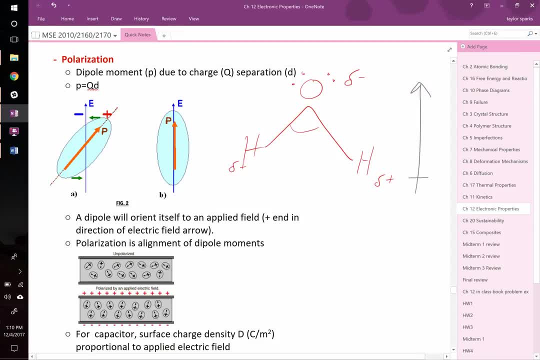 like this. We say that its dipole looks something like that. right, This molecule, just as it exists, every single molecule of water- is polar, meaning it's got a North Pole and a South Pole. right, It's got a positive charge and a negative charge here. okay, So this? 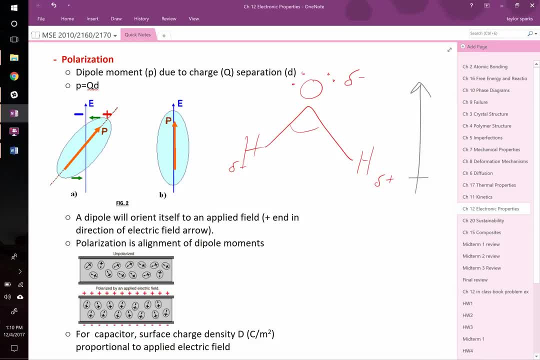 has a built-in dipole moment. Not all molecules have a built-in dipole moment, Some of them. you have to, Yeah, to induce a dipole moment by applying an electric field, right? if it does have one. imagine if this is in the presence of a parallel plate capacitor, right? so here's. 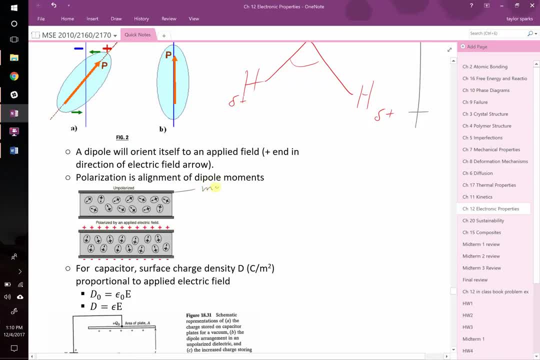 our parallel plate capacitor. we've got our metal at that point and at that point. but in the middle you have a polarizable molecule, molecule with a dipole, right, if you don't hook a battery up to this thing, then there's no reason why these poles would all be aligned up right. they might generally kind of be. 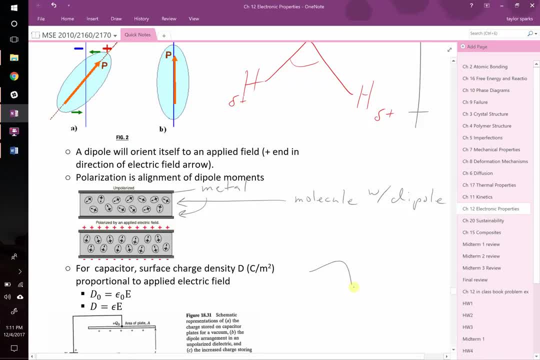 doing something. hydrogen bonding- right, we know that water molecules kind of like to nest a little bit because hydrogen bonding, but there's no reason they all have to be lined up the exact same way throughout this material. right. that changes when you apply a voltage. when you apply a voltage, this thing 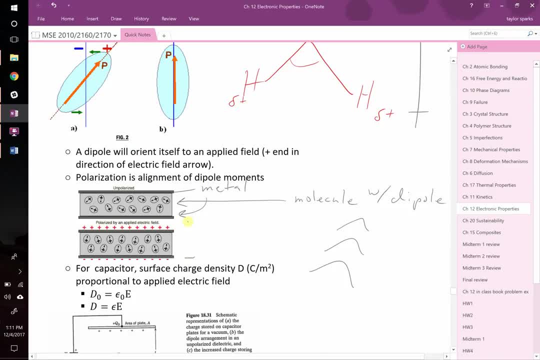 let's say that we put a bunch of electrons on this bottom side. we put it, we take away electrons from that top side, right? so you've got this negative and positive charge thing going on all of a sudden. all of those molecules that are within here, they're going to react to that right, because 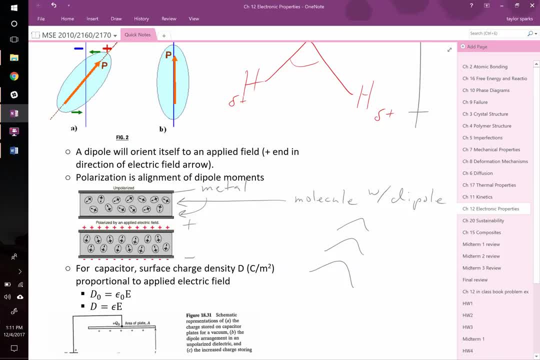 you've got this negative charge here, the positive of these molecules is going to be attracted to it. because you've got positive here, the negative side is going to be attracted to those right. so the fact that your material can donate its dipole to the applied voltage to allow you to store even more, there is why is why we 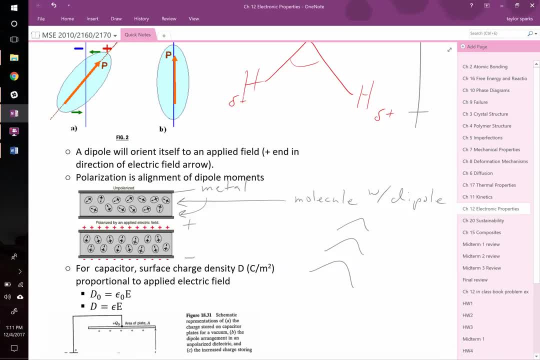 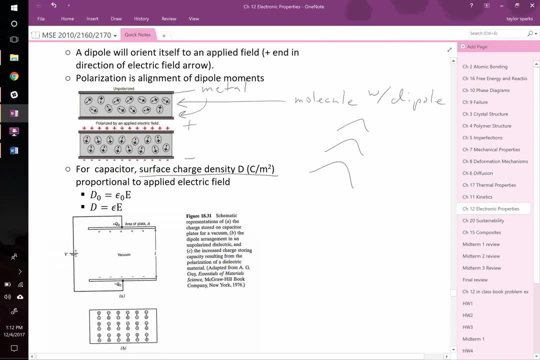 can store more charge when there's something in between it, between rather than just two parallel plates. okay, so we call d the surface charge density. again, that's going to be the charging accumulate. forget some given surface. so, per meter squared, for example, how much charge can you put on something that's deep? and again, if you had 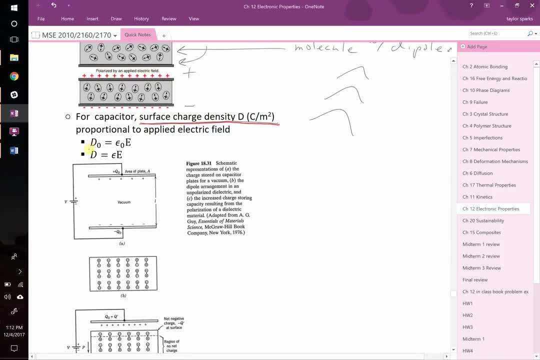 nothing, they're just vacuum. then the surface charge density would just be proportional to the electric field and the permittivity free space. but when you put something there that's a dielectric constant, it become its scales with it. basically it's a one-to-one ratio. 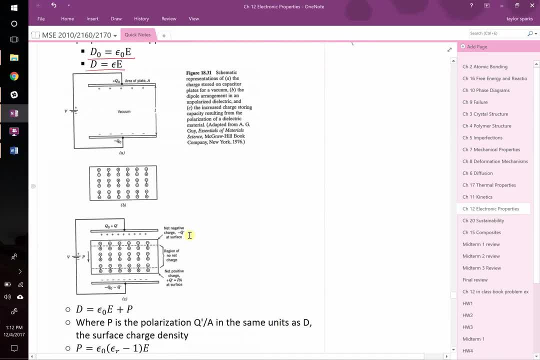 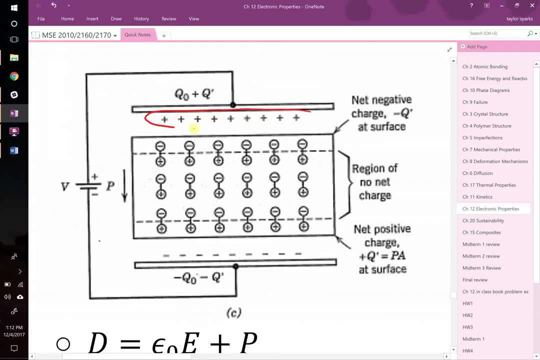 scales with it. okay. so again another example of this. here they show a big dielectric material. you've got say this is some sort of ceramic, let me make that bigger. you apply a positive charge up here, right, and the ceramic might be able to orient itself if it's an ionic material. 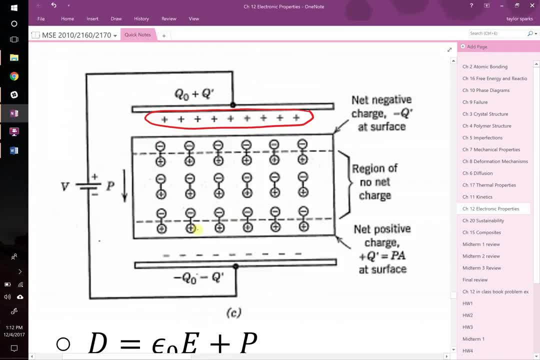 where the negatives might arrange themselves on this side, the positives might arrange themselves on that side. if you look within the bulk of this dielectric material, none of that is doing you any good, right. all of those charges, cancel out, right? they're not adding on to your dielectric moment. 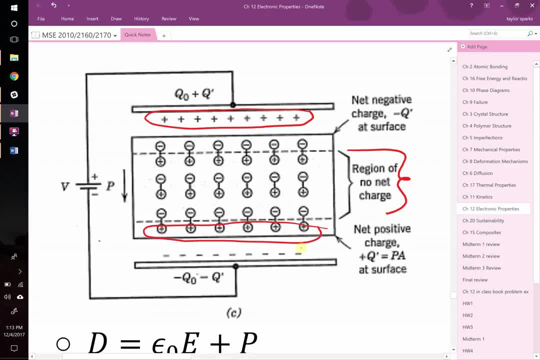 but all these ones here, these do let you store more electrons on this surface, right, so your dielectric material doesn't have to be thick. it's not like if you make it really, really thick, make it a centimeter thick, you're going to make a better capacitor. no, just the opposite, because 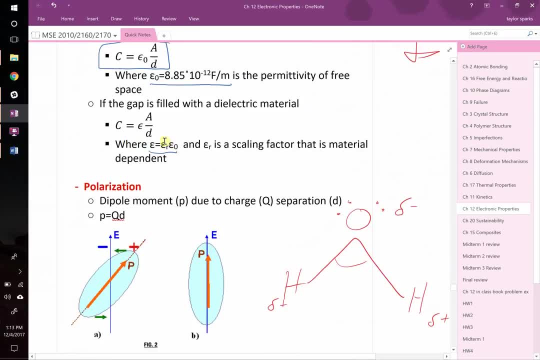 just like before. we know that capacitors get better. the thinner you make them right, the smaller this lowercase d value is. you're going to make a better capacitor, the better your capacitor is, and all you need is just like that top and bottom layer of your dielectric material anyways. so it's in your favor to make it thin, but to put a very thin layer of. 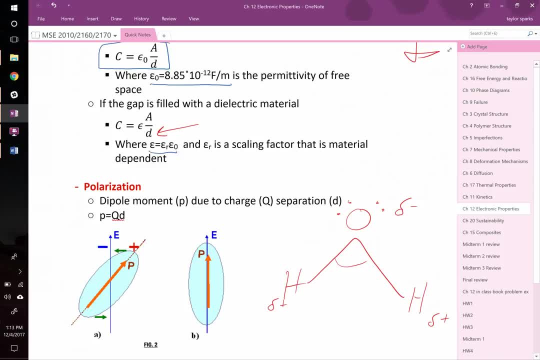 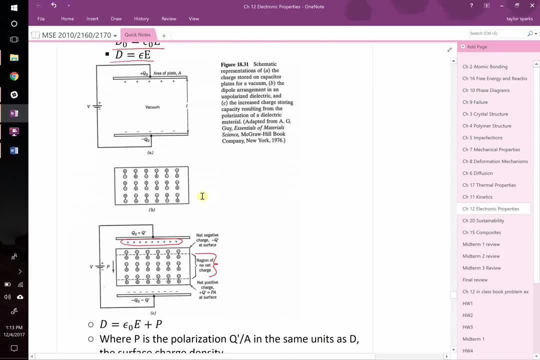 your dielectric material in there. any questions so far on this, on these charges where they're coming from? no, so again, just comparing these two cases, you might have looks like they put like five positive charges here because this was just under vacuum. by the time you put something in it, they've. 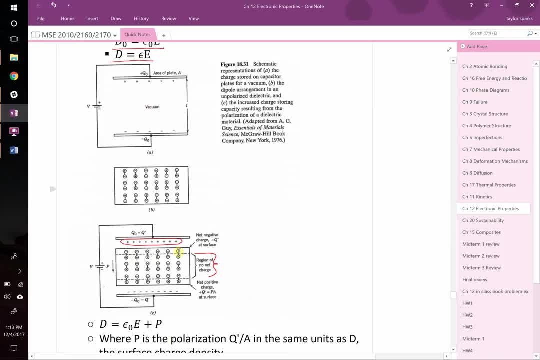 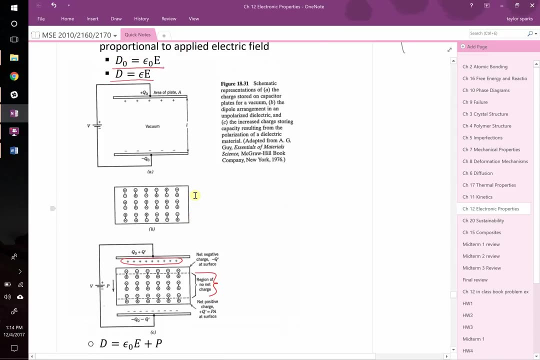 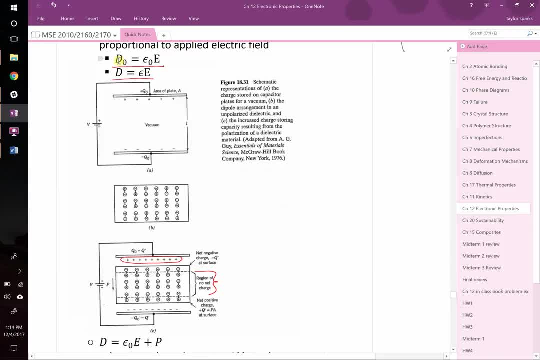 whatever charge it is, it's going to be some charge. it's gonna be proportional to your electric field, right? we haven't. d0 doesn't have like a value you could calculate based off of your field, right? because e not has a document that says all of this is a product of double the невw, which it's. 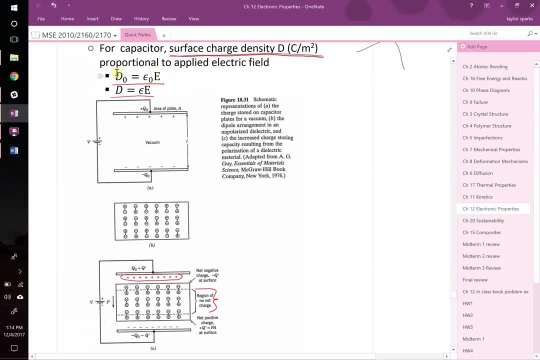 is a constant. epsilon, naught is a constant. so with your electric field, d naught is going to increase and then you've got that same thing, but now you've got a dielectric material, so it's going to increase where epsilon. recall that epsilon is technically equal to epsilon r times epsilon. 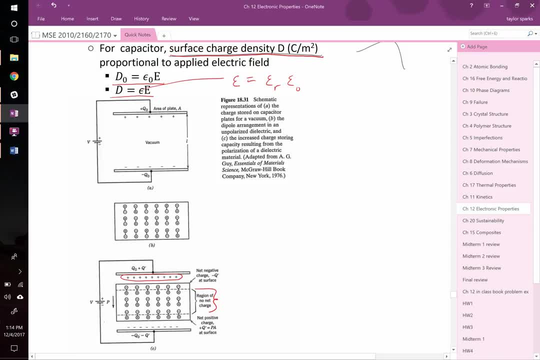 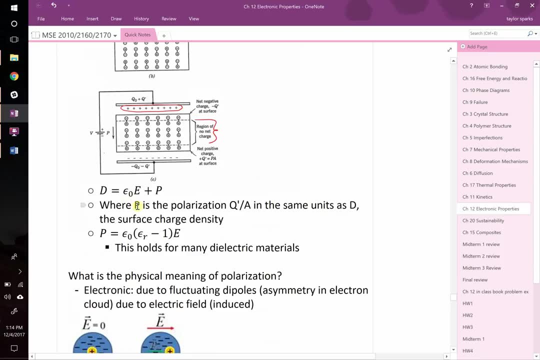 naught. epsilon r is just a number. epsilon naught is the permittivity free space, right? so there's those two, and then down here they show an estimation, right? so p is what's called your polarization. that is, in charge per area, same as in d right, and polarization can be roughly. 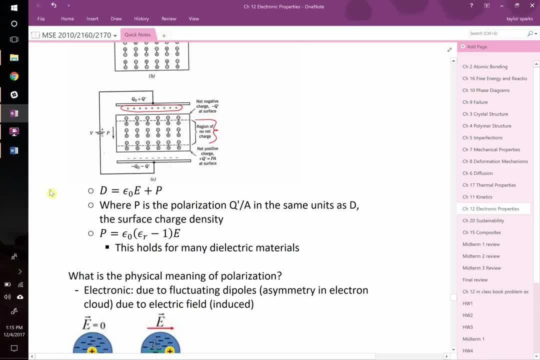 calculated for some materials. that's what this third expression is basically says: okay, whatever would be for a vacuum, plus this extra term which we're going to call polarization, and the way that we calculate polarization is with this right here, basically permittivity, free space times, this, this. 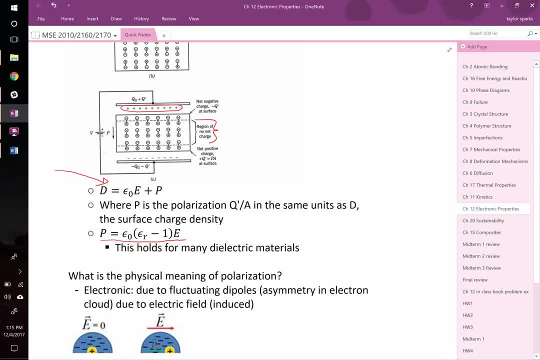 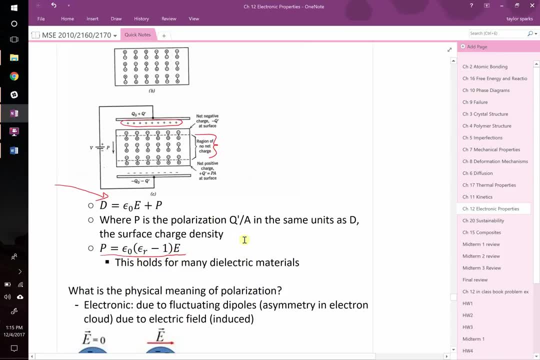 quantity of epsilon r minus one that all times e. that's going to hold for some materials, all right, so yeah, so polarization does relate to voltage. this is polarization here, and electric field that's related to voltage. remind us how does electric field relate to voltage? yeah, in this class we've been doing more simple. that's the physics definition. it's just. 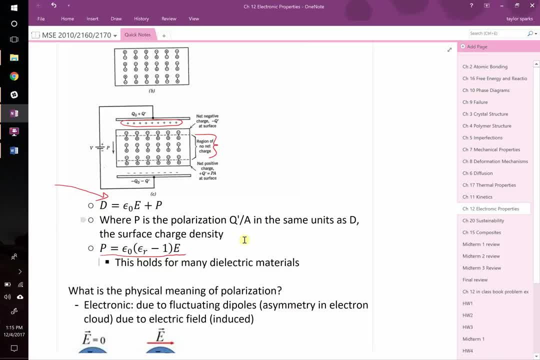 the, the separation, right. if you've got two leads from a nine volt battery and you separate them far apart, then you have a small electric field between this. you bring them close together. your electric field is large for the same voltage, right? so that's how voltage comes into place in your electric field. it's dv over dx, basically. 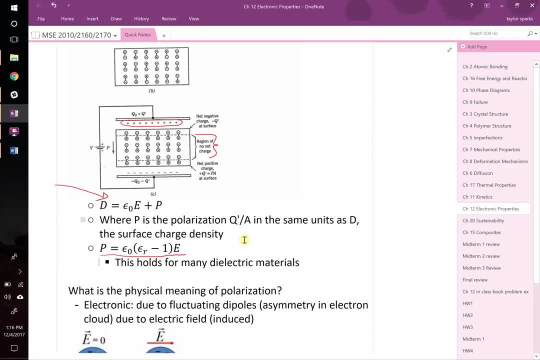 right, okay, other questions? so far okay. so where does this polarization come from, since this is like an easier expression to use, um, where is this polarization coming from, right? so polarization can come from a number of sources. in fact, it never comes from just one thing usually. it's usually a. 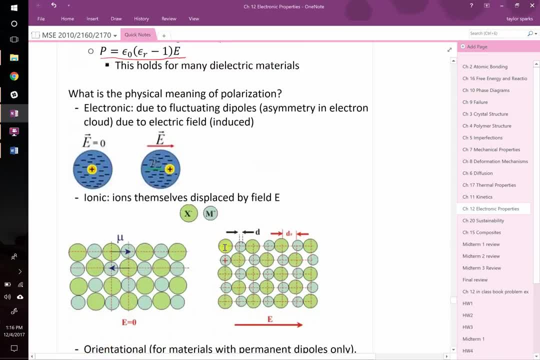 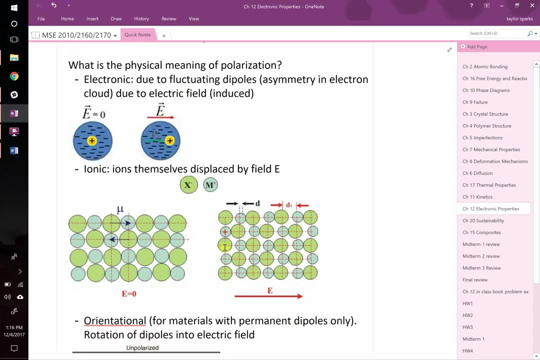 contribution from several sources. so the first thing that we're going to consider is the electronic contribution to polarization. electronic is literally what it sounds like. you've got an atom which has maybe lots of electrons. take lead. lead is number, i don't know what- 70, 80, 90. it's got a. 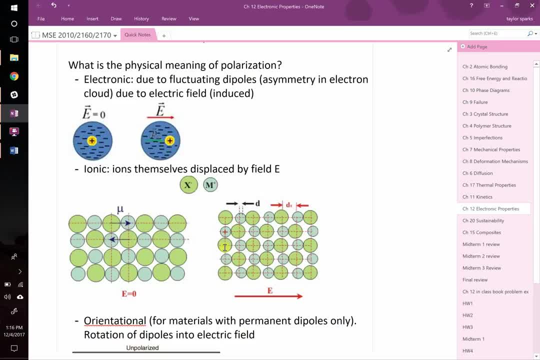 ton of electrons and if you apply an electric field to that thing, on average all of those electrons might shift to one side a little bit right now, as soon as you take that field to the way they're going to go back. but that's not the point. the point is that when you apply a field, 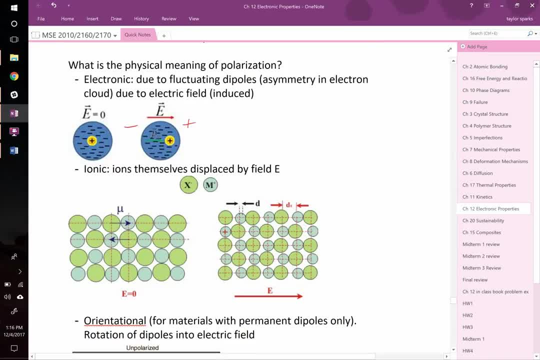 you make this thing net negative on this side and net positive on that side. right, therefore, if your material was this, as long as it doesn't connect electricity, that would be a dielectric material. right, because you can get some dipole moment out of it and therefore you increase the amount of 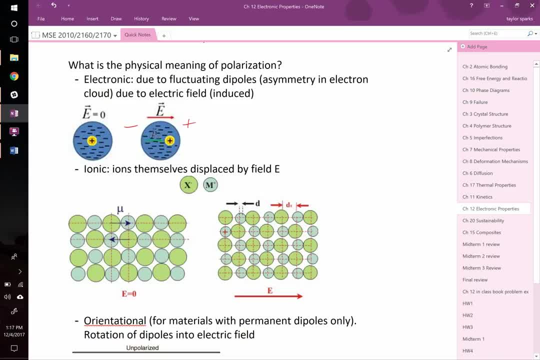 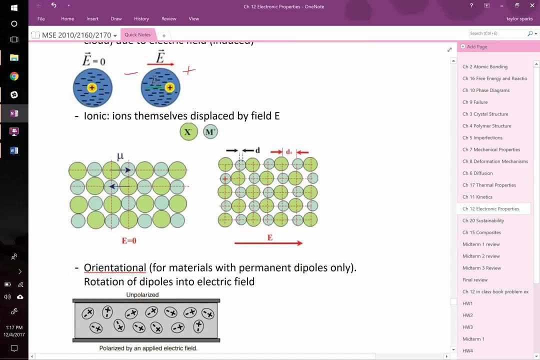 charge. you can put on the surface any questions. yeah, rosa, um, how, how do you like in ceramics? okay, move over each other. yeah, so that's a great question. that leads us to our next one. right, the? so we had the electronic contribution, which is literally the electron cloud. 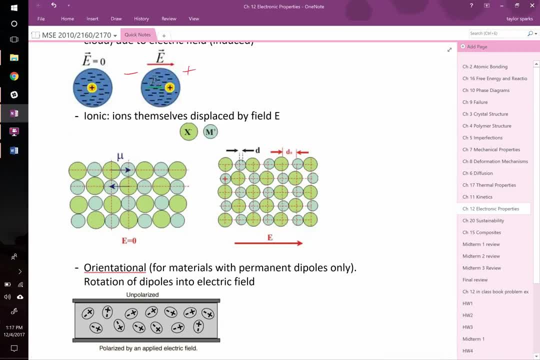 shifting a little bit. right, we know where it wants to stay. normally it can shift a little bit, especially under a field, now ionic. this is when things actually move right. so you apply an electric field and this is your material. you've got these two molecules right. they've drawn the 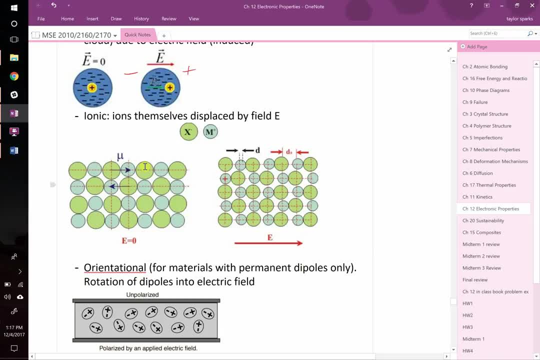 smaller one is the cation, the larger one is the anion. and when they apply an electric field to this thing, in an electric field the positive things want to move that way and the negatives want to move that way a little bit. so you'll see that your anions have shifted a little bit right relative to your. 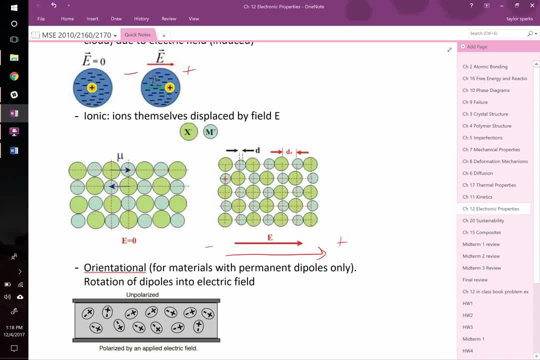 patterns, so your cations will literally shift a little bit over in your hands. a little bit over that might. um, that's going to break the symmetry of your crystal structure, right? this may not be the same crystal structure before and after applying the field. it might change it from cubic to slightly tetragonal, for example. but that's okay, that can. 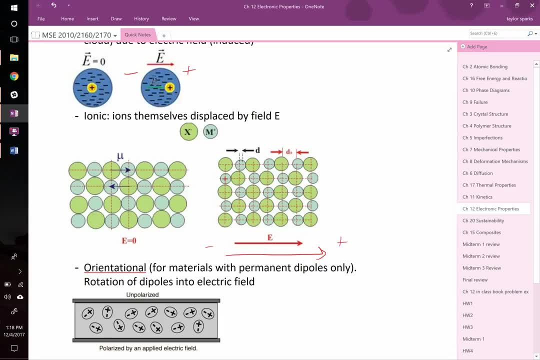 happen. so atoms can shift a little bit. um, typically, these aren't huge amounts that they shift, it's like fractions of an angstrom, but they can shift a little bit and in doing so you build up negative, positive, you're, you're able to store more charge on the surface. okay then, um, there's orientational. 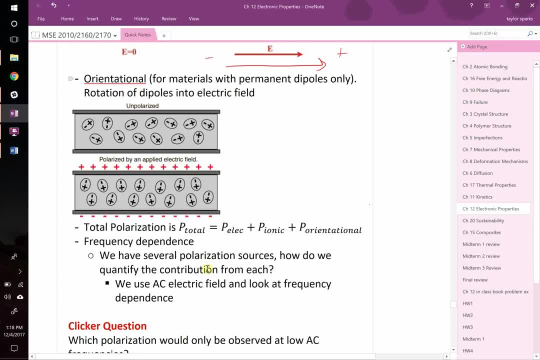 this only works for molecules that have a permanent dipole, things that you can rotate them and then, no matter what you do when you rotate they still get a dipole. you can just make it line up to your field. so water- right, you can take water which is sort of random all over the place and then 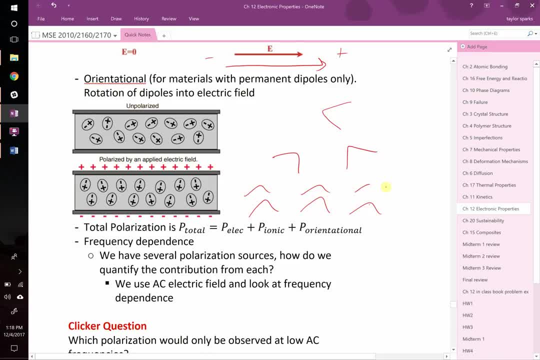 when you apply a field, you basically make it line up and in doing so you can put more charge on the surfaces. so those are the three that we're going to talk about: electronic, ionic and orientational right. so we're actually done with clicker questions for the semester. huzzah right. 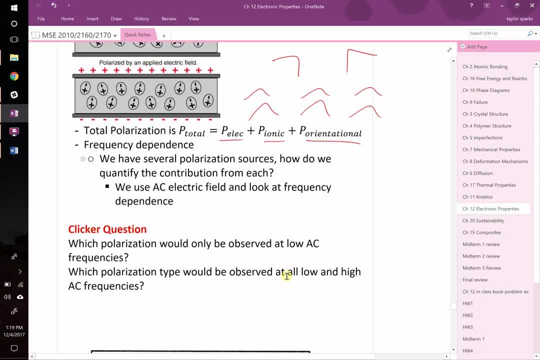 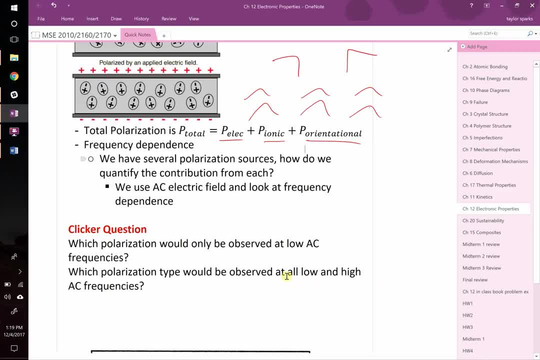 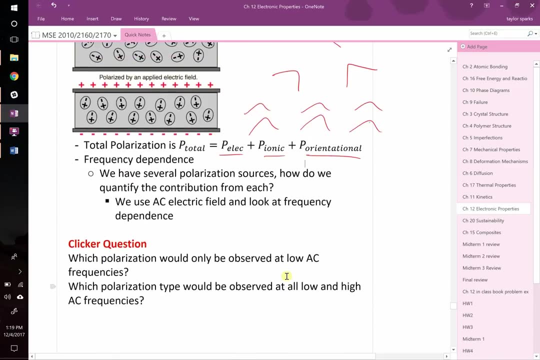 alternating current right. so that's, your voltage goes from positive 120 to 0. positive 120 to 0 keeps on switching. think about how that, how these different sources of polarization are going to respond, right, if you sketch them as a function of time, how are they going to respond? which ones will respond fast? 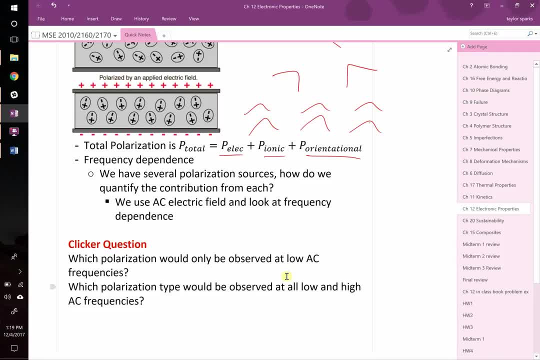 slow. you know, kind of, in between, discuss that with the neighbor, right? okay, so let's discuss this, and I'll do so using a volunteer. well, actually, let's. let's ask somebody first, like which one should respond to low frequency versus high frequency. any anybody have thoughts on this, right? what do you think? 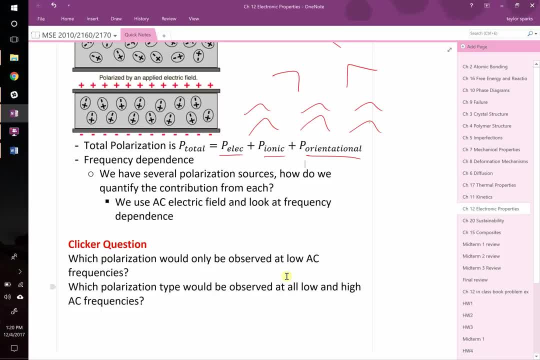 I: yeah, bingo. so, Kevin, can you come up and illustrate this for me? Kevin's going to help us out against his will. what I'm going to do is he's going to take a big step. he's going to represent like a molecule shifting in the presence of an applied field. so every time I'm 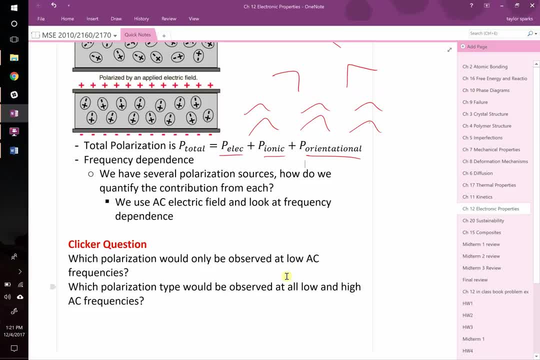 going to raise my hand from this way to that way. when it's this, you're going to take a big step. that way, right, just like that. when I go this way, you're going to go the other way, so let's do first this, exactly right, no problem guys. up, all right and up guys. 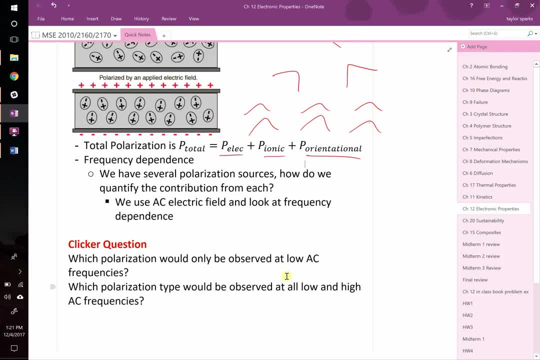 one as well. right now you can't keep up right. there's literally like some, like mechanical across that they can't go faster than that. making it important for them, right. so some things: if it's like a whole atom that has to diffuse, like migrate, like from one side of the other, it has some limit to its speed. 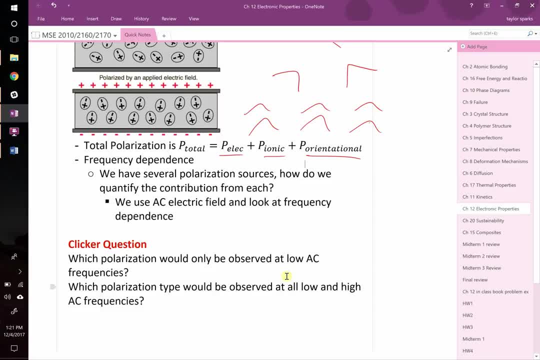 If you're talking about electrons in a cloud, electrons are going to be able to shift really, really quickly, And if you're talking about a whole molecule that has to rotate, it's going to be the slowest of all. So if you look at the frequency response, 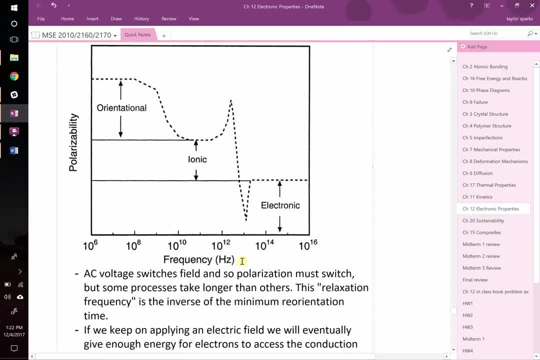 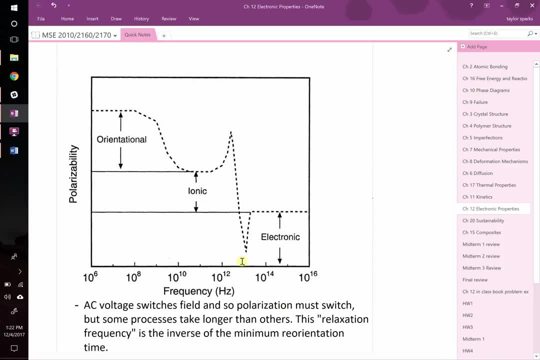 of your dielectric material, you typically see curves that look always like this: right The y-axis is your polarizability. Polarizability is: how much dipole can you accumulate? by whatever means all three of these right is possible. right, This is versus frequency, So high numbers. 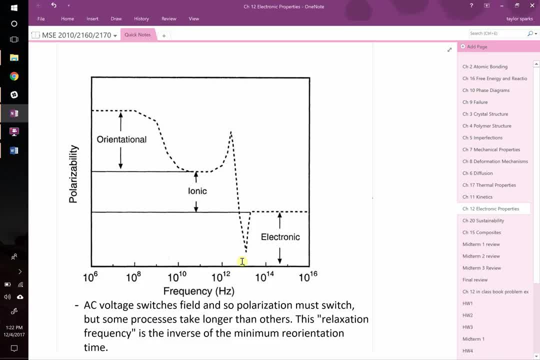 of frequency, that's many times switching per second right. So if you're switching at something like down during the 10 to the 6 frequency, you have all three of those. things can respond. It's slow enough going back and forth that the molecule can rotate, it can shift, the electrons can move. 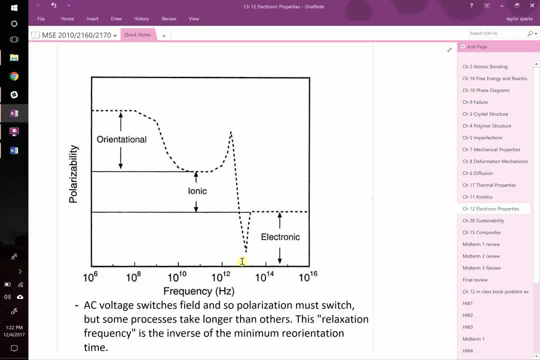 no problem. If you speed it up into this middle regime, then only ionic and electronic can respond. Speed it up a little bit further and you've only got electronic right. So a dielectric is not like a constant number. It really depends on the frequency that you're going to use it at. 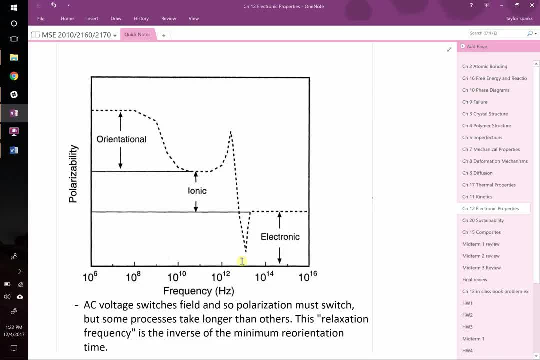 Right. So if you only ever care about the frequency in your home right, which is 120 hertz, then that's way low compared to these. You can assume all three of those are going to be present, right? But if you're doing high frequency electronics you can actually use. 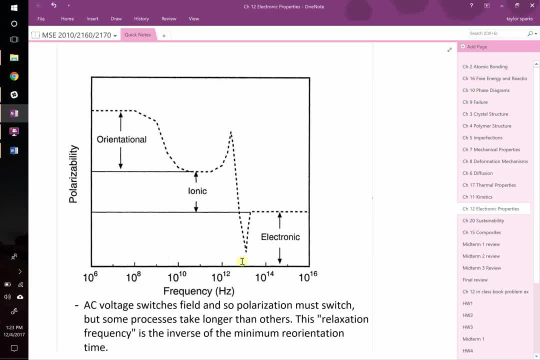 this. You can make filters out of it, right. So the filters that filter out, say, low frequencies versus high frequencies for music, right. If you want to have like tweeters versus subs, right, You need to filter that. You can do something like this that will filter it where there's literally. 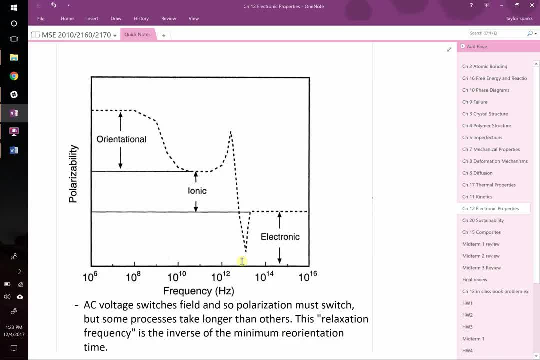 no frequency cutoff where something can't happen, And you could use that to filter out high versus low frequencies. Yeah, And that's not the only way. That's one way, Josh. So what's happening in between here is beyond the scope of this course. In the class I used to teach 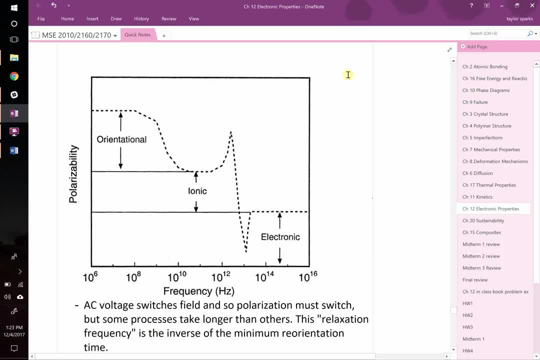 in ceramics. we'd get into it In other courses. you will see it. Basically, what you have at these transition regions is what's called loss: You actually get heat generated. So this is exactly how microwaves work: You get heat generated, You get heat generated, You get heat generated. 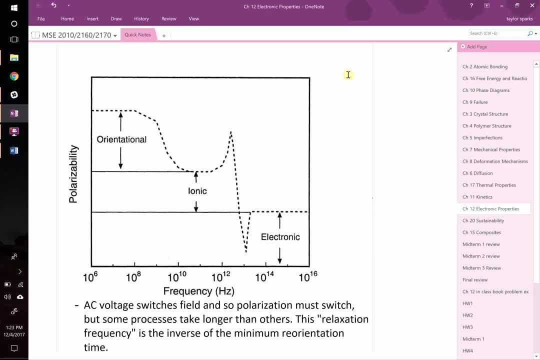 Right Microwaves, you have water, which is a polarizable molecule, And you've got incoming radiation from your microwave And if you pick the right frequency you can actually pick it right at one of these transition points between where water molecules rotate. I'm pretty sure microwaves work. 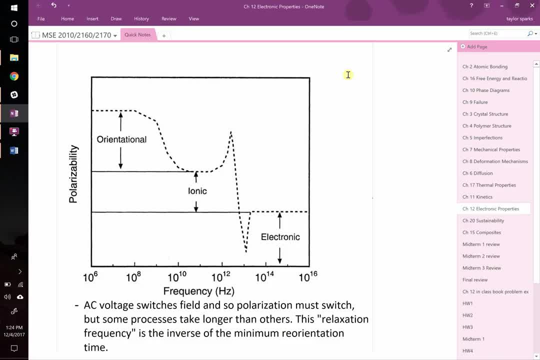 right here. I could be wrong. I think it's right there, though, And because you're causing them to want to shift back and forth, but they can't quite keep up with the speed. you generate a ton of heat Right. You get loss. You get dielectric loss, which is heat generation. 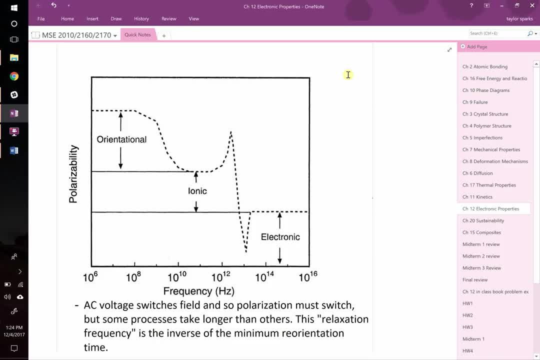 Again, that's beyond the scope of this class, but that's kind of what's happening at these intersections of these different regimes. Okay, Other questions? Anything on this? on the frequency response: Super easy test question to ask. Give you this curve, ask you to explain what's going on in a 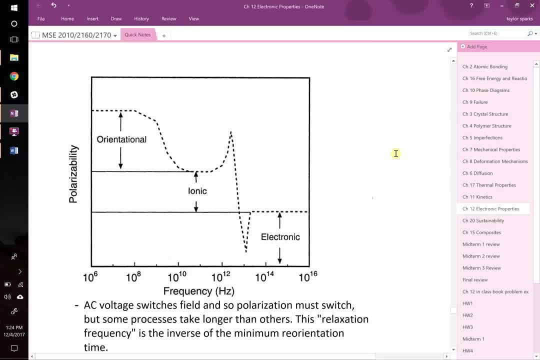 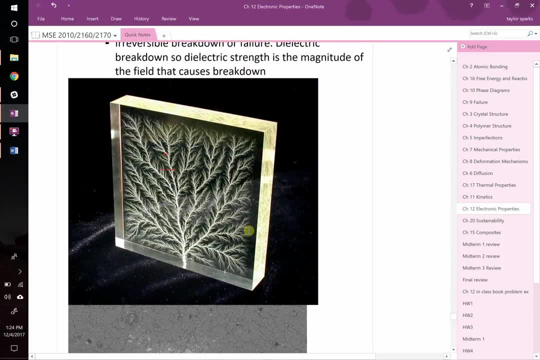 model material, Right, Okay, So how about this? Let's say you've got a material and you apply a voltage, right, And for however thick your material, the bigger your voltage, the bigger your electric field, right, Because the thickness isn't changing. now, 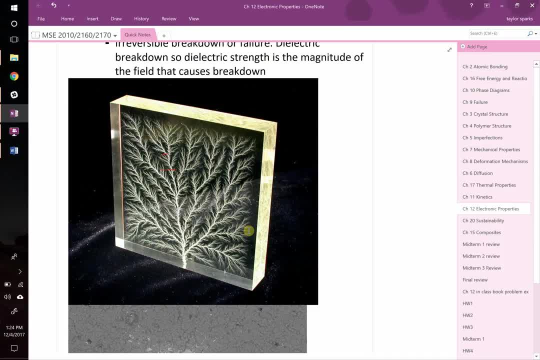 Just your voltage is getting larger and larger and larger. At some point, if you keep on increasing the voltage, you will get what's called dielectric breakdown. It stops behaving like a dielectric, meaning it's producing charge on the two surfaces, but no conduction, no current, And all of a sudden it conducts electricity. 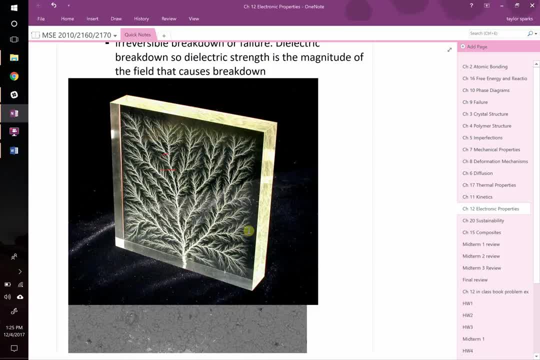 in a very big way, right, It actually all of that current rushes through your material. It locally melts it and destroys your material, And it usually is a point of failure. Some things are designed to make this happen, right, But almost in all cases this is something that causes failure. So here's an example where they induced dielectric. 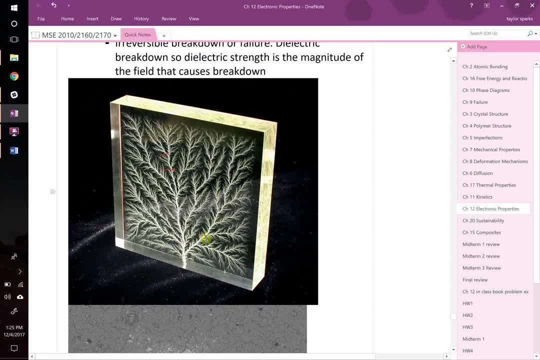 breakdown in this piece of glass or acrylic or whatever it is right. They applied a voltage right here, right Like a point source of voltage. They hooked a multimeter or something up to it. They must have had all along the other. 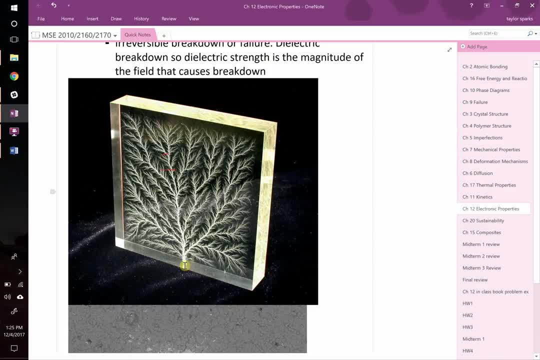 three sides. they must have had something like copper tape that was conducted to complete the circuit. They increased the voltage higher and higher, Until they caused the electricity to arc its way through the material and create this interesting sort of lightning type pattern. When you see lightning in the air, that's exactly what's happening. You've got your clouds, which are accumulating. 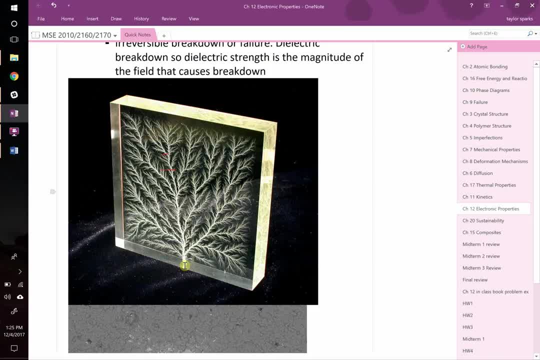 charge relative to the ground below. The air itself is not a vacuum, So it's going to have some dielectric constant. that's better than vacuum. If it with different moisture levels, that all changes right. But at some point if you get a big enough, 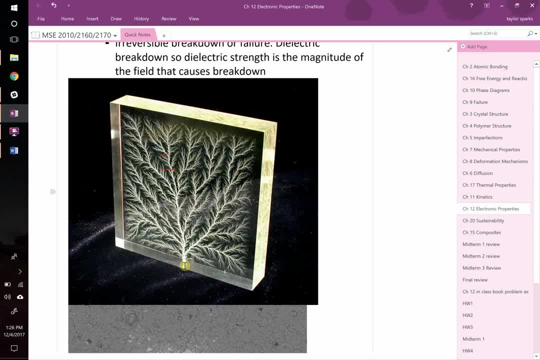 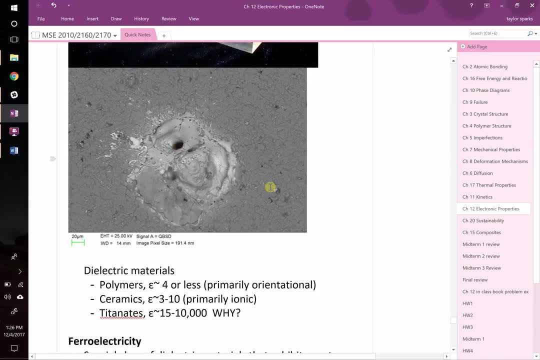 charge accumulation. then your electric field gets too big. You're going to arc across it and that's lightning right. In electronics it looks like that. It's a small spot. This is about maybe 5 to 10 microns big. They just got locally melted. 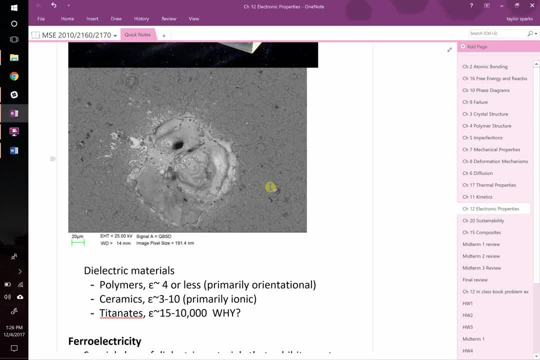 completely. It's like a tiny little lightning bolt just shot right through your material, destroying your component right. So dielectric breakdown is something that is usually to be avoided. You might be designing it so it's like a failsafe before voltage gets too large. This could be like how a fuse blows, for example. You could induce it to fail at a certain point If you knew the. 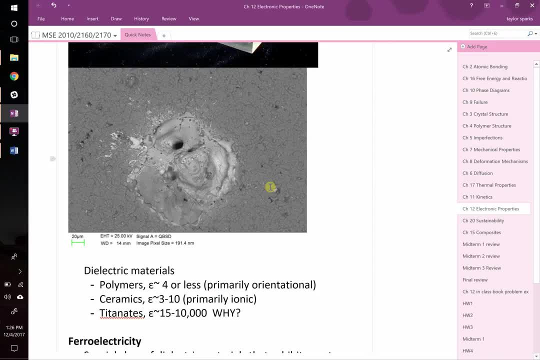 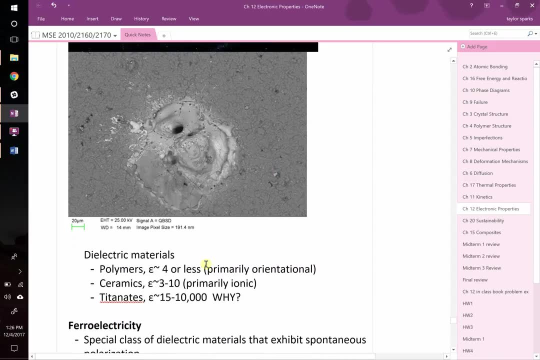 dielectric breakdown field of your material. Yeah, Is this how this is working? I don't think so. Maybe I don't think so, though I'd have to check on it, I don't know offhand. All right, So let's talk about- we've already said this a little bit, but dielectric constants from. oh yeah, Thomas. 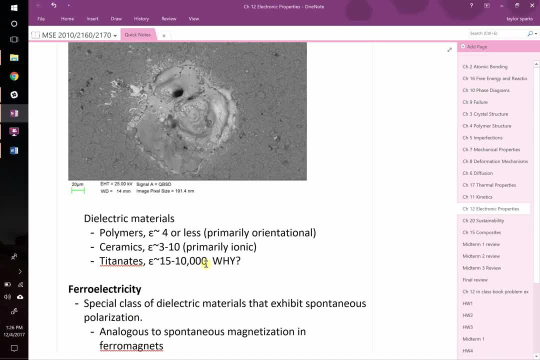 How are non-polar molecules? how are these non-polar molecules? How are non-polar molecules? You're going to see an example in just a second. So hold on to that thought. Basically, you can't rely on the rotational aspect. You've got to rely on ionic and electronic. And ionic becomes really big in some cases. Okay, 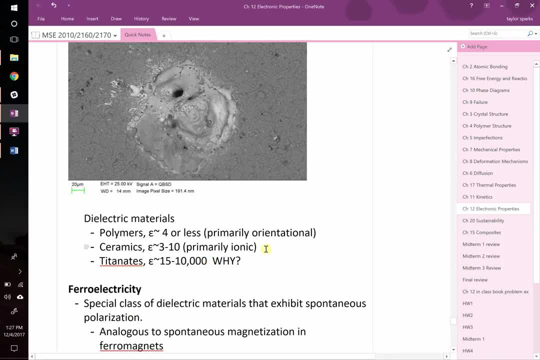 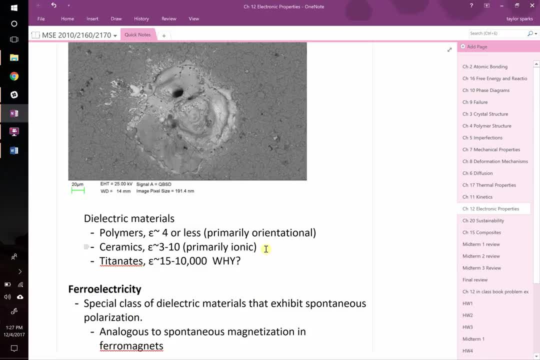 So they don't have a very high dielectric constant. Most ceramics these ions are pretty tightly bound and they don't want to shift and move in the lattice. It's a pretty tight lattice to start with maybe, So you don't get a lot of dielectric constant there. But in some ceramics- the titanates and the zirconates and a few others- you can get just bonkers numbers. You don't get a lot of dielectric constant there, But in some ceramics- the titanates and the zirconates and a few others- you can get just bonkers numbers. You don't get a lot of dielectric constant there, But in some ceramics- the titanates and the zirconates and a few others- you can get just bonkers numbers. You don't get a lot of dielectric constant there, But in some ceramics- the titanates and the zirconates and a few others- you can get just bonkers numbers. You don't get a lot of dielectric constant there, But in some ceramics- the titanates and the zirconates and a few others- you can get just bonkers numbers. 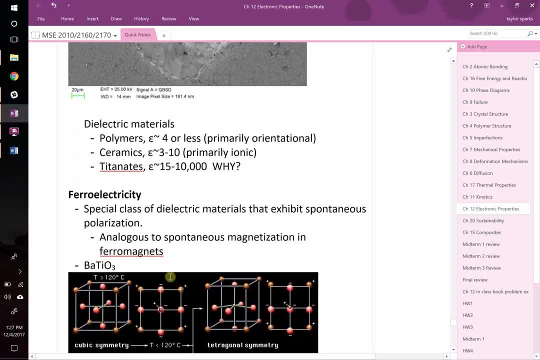 You don't get a lot of dielectric constant there, But in some ceramics- the titanates and the zirconates and a few others- you can get just bonkers numbers. The easiest way to explain it is to return to our crystal structure that we love the most. 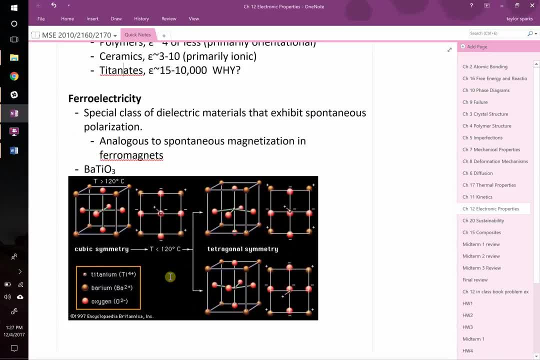 the perovskite right. So we're going to do so and explain it, while simultaneously explaining something called ferroelectricity. So ferroelectric materials, these are a specific class of materials that have a spontaneous coupling between- well, basically a spontaneous 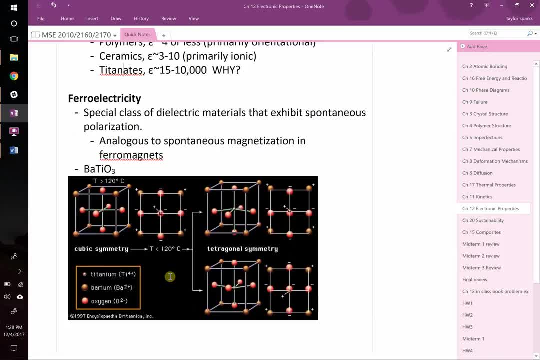 polarization. I should say So. an electric polarization automatically occurs in these materials. when you change their temperature Above a certain temperature the material might be cubic. So in this material this is probably barium titanate. Yeah, barium titanate at 120. 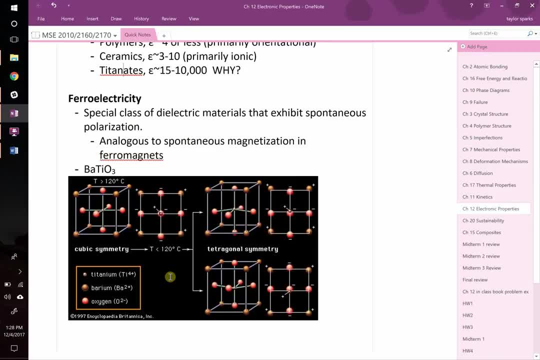 degrees C and above, you're cubic. If you look at this, there's no dipole here. So whoever was just asking that there's no dipole in this molecule? So if you were to make a dielectric out of this and say it's not going to be great, what happens is that below this temperature, 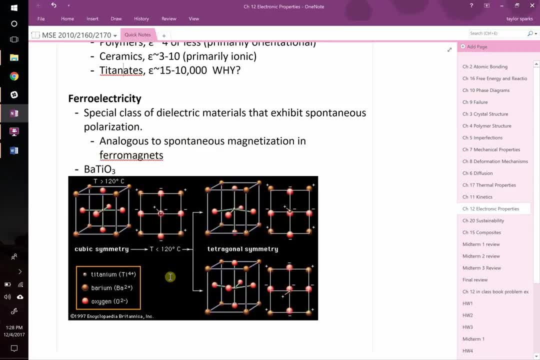 which we call ferroelectricity. there's no dipole in this molecule. So if you were to make a dielectric out of this molecule, you could call the Curie temperature, by the way, The temperature where this transition occurs at 120 degrees in this material. that's the. 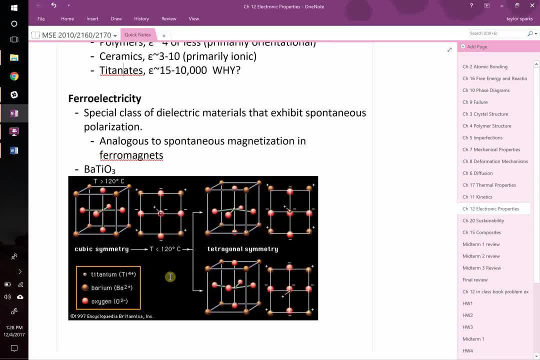 Curie temperature, not Curie right. What happens is that below that temperature it shifts from cubic to tetragonal. The way that it does, that is, the lattice gets a little bit taller in one dimension and these atoms actually shift a little bit right If the 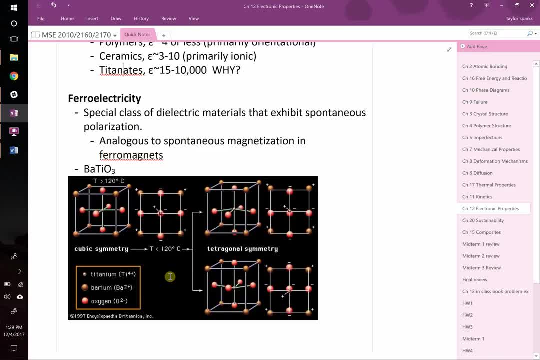 field is one way versus another. you're going to have this positive ion in the center. That's your titanium ion. That's titanium four plus, by the way. So that's actually taking a lot of charge with it. It's going to shift down. Your oxygen is going to shift. 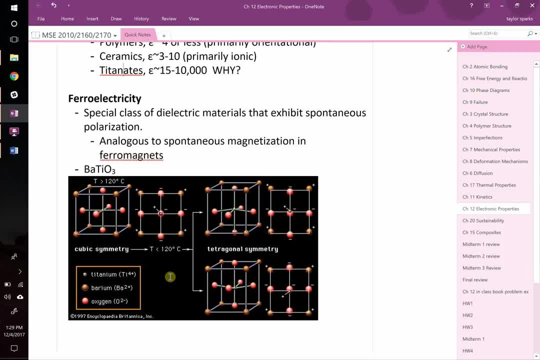 a little bit up, Your barium is going to shift a little bit down. So in this molecule these are barium two plus oxygen, two minus titanium, four plus All of those atoms are shifting just a little bit. To do so it broke the crystal symmetry right. Clearly this sort 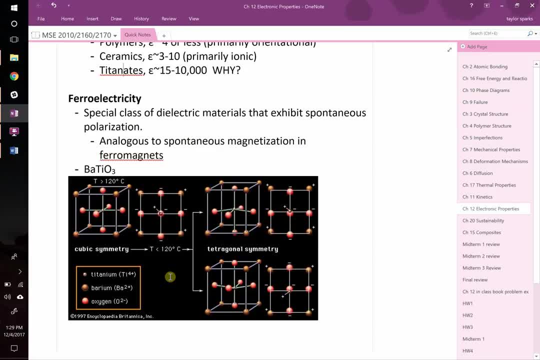 of capacitor is only going to work effectively below its Curie temperature. If you heat this thing up above 120 degrees it's going to shift a little bit. So if you keep this thing up above 120 degrees it's going to shift a little bit. So in this molecule these are 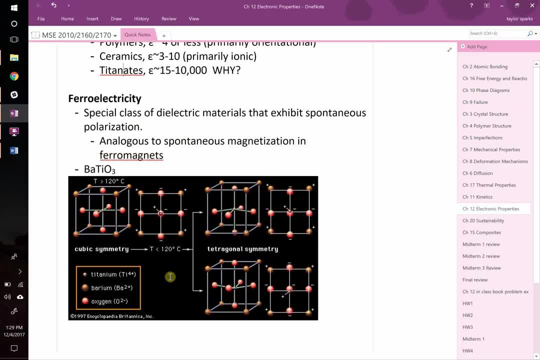 Seems on average. it looks cubic. So while it might be temporarily polarizable, it's not going to stay that way. These ones are interesting in that they spontaneously occur and they stay that way. If you take this crystal and cool it down, no electric field. 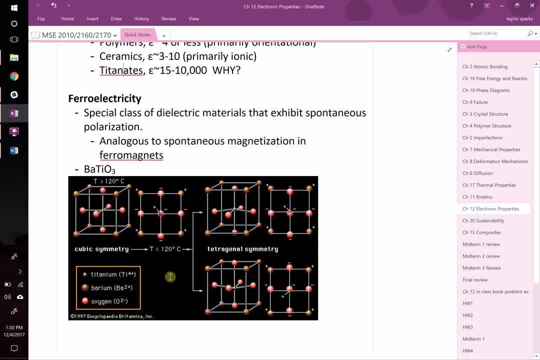 needed. all on its own, These atoms will shift a little bit right, For reasons that won't quite get into this class. They're going to shift because it lowers their energy slightly, right, And then, now that it's shifted all its own, you can switch that shifting right. 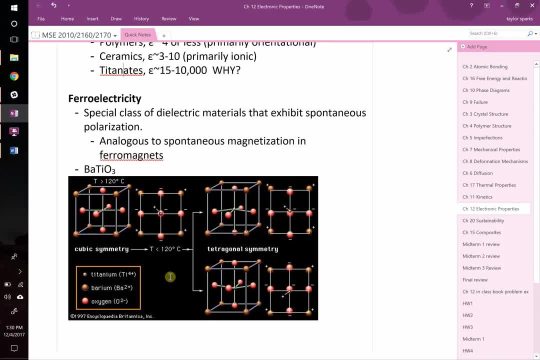 If I apply an electric field the opposite way, the Kraken weight will be one volt right For my falsification. Here's my crazy amazing to ask the question: Tell me what direction this titanium, instead of being shifted down, it's going to shift up, and the 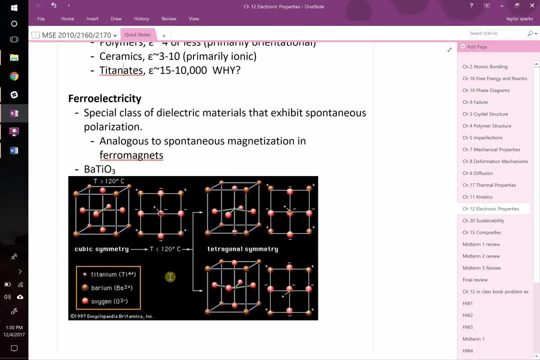 oxygen will do the opposite. right, So you can switch this back and forth, which is great, because that's exactly what we want in our parallel plate capacitor, right, When we line this thing up, all we want is that something, some sort of molecule, can create a negative 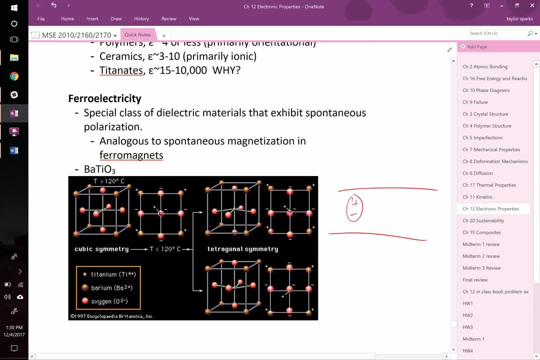 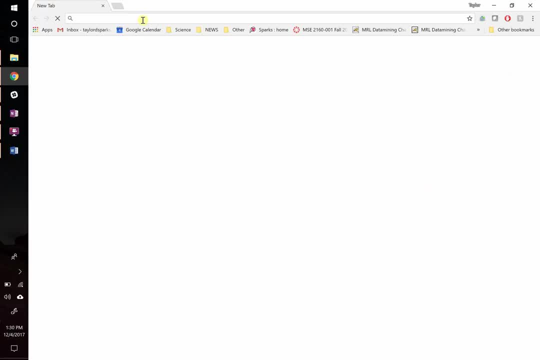 and positive, And because your titanium atom has a four plus charge and it can move quite a bit, you get a really big polarization. So I saw a hand, just one second. let me show you this. So let me pull the crystal structure really quick here. They'll often show it like 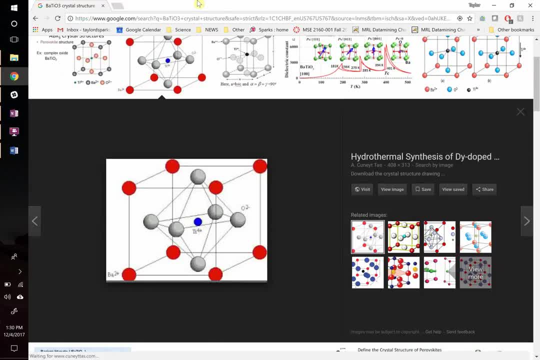 this with a polyhedra around it. right The octahedra. And the smaller this titanium atom is relative to the size of the cage around it- the oxygen ions- the more that titanium can shift. So I don't remember who discovered this, but somebody. 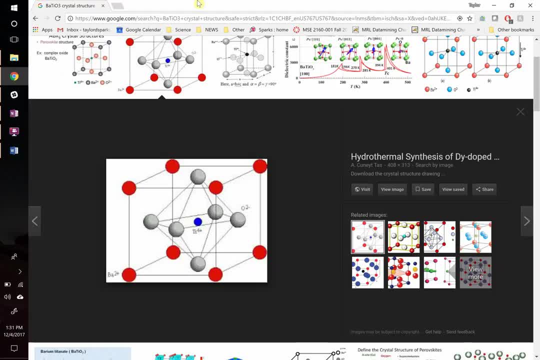 you realize that titanium is a pretty small atom relative to the cage that it's in. Therefore it can move quite a bit when you apply a field And therefore you get just enormous polarizations, like 10,000 times larger than what you'd expect in other materials that are similar bonding. 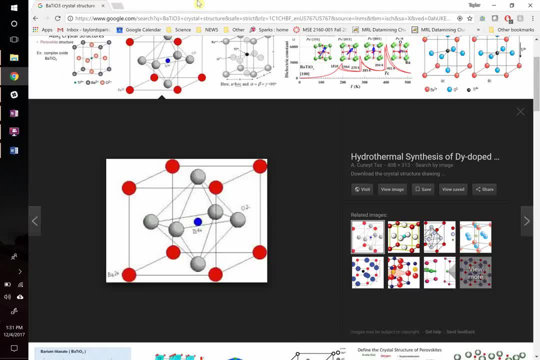 similar type of atoms but don't have this structural feature that allows for really big polarizations. Now again, all of your atoms contribute to the polarization, but titanium is the big one because it has the biggest charge and it moves the most, So it's the real big contributor. 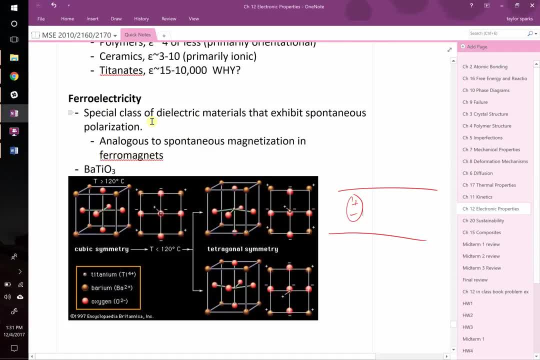 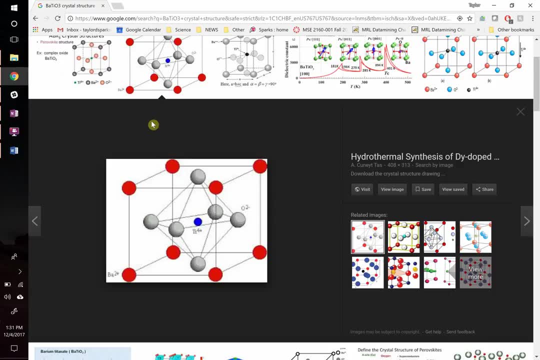 Any questions so far? Yeah, Rob, One about the other time. I just noticed this. a little question popped into my head. It says that it's dysprosium doped. Why would you put dysprosium in this? 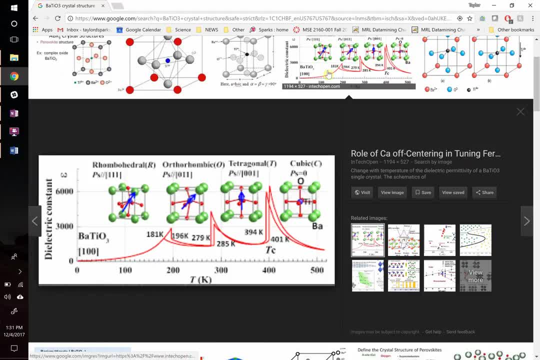 The reason that they dope them, to my knowledge, is because I had a postdoc stay in my group for a while. Basically, as you dope it, you can change the temperature of that transition. Remember, at high temperatures it's cubic and then it switches to triagonal lower temperatures. You can basically 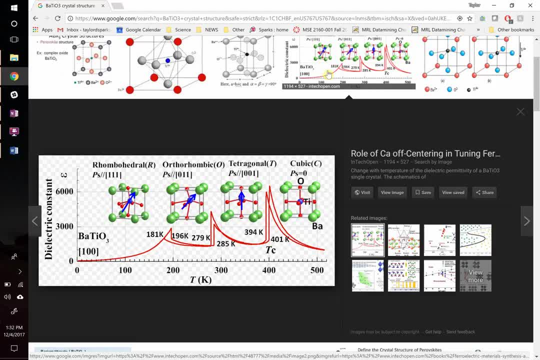 move the temperature at which that happens. You can move the temperature at which that happens. You can move the temperature at which that happens a little bit by doping it. To my knowledge that's why they do it. There could be other great reasons that I'm not aware of. Other questions? Yeah, in the 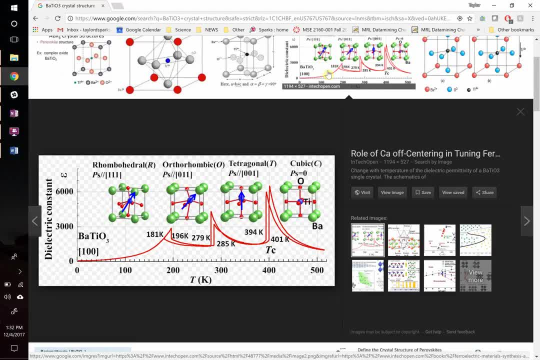 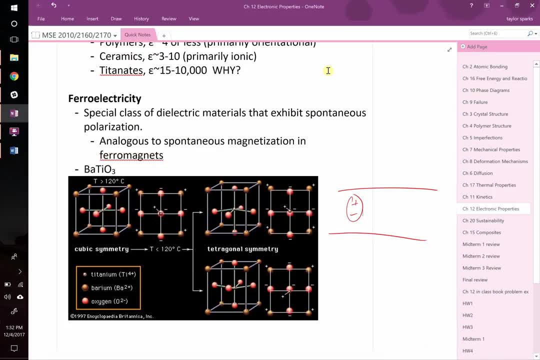 back Landon. I have a question about ferroelectric and ferromagnetic. What is that ferro? what does that say? Yeah, so the origin comes back to when they first discovered magnets. They knew that ferrous materials which were loaded with iron were magnets. So this is actually the next thing. 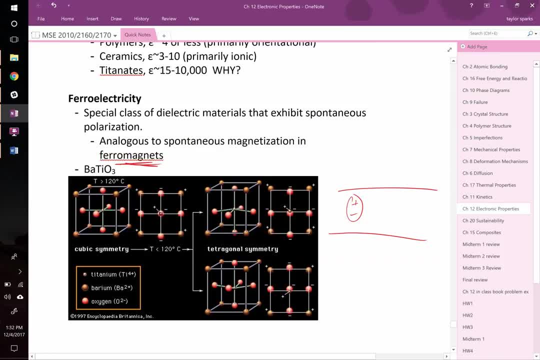 we're going to talk about, And magnets, ferromagnets like lodestone, magnetite, which you can dig out of the ground, which is what, early in the early days, they did. They had this rock, They knew it was ferrous. 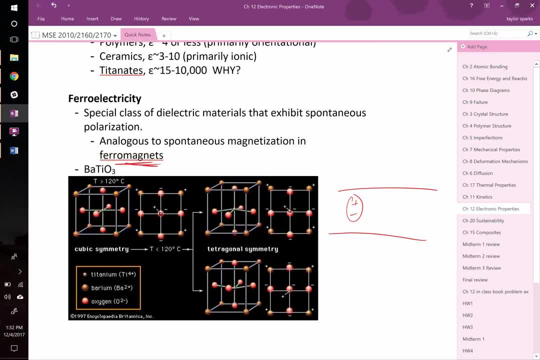 because they could melt it down and make iron out of it. But this rock itself was magnetic, right? Iron filings would stick to it, right? And in that case we're not talking about an electric polarization. In that case there's a temperature above which it's not magnetic and a temperature. 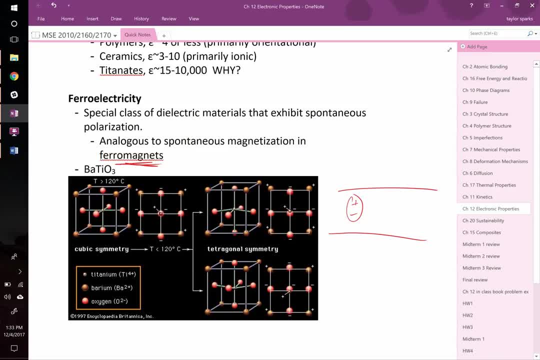 below which it spontaneously magnetizes. If you remember our iron wire demo forever back two months ago, we had the magnet sticking to the wire And when we heated it up it spontaneously lost its magnetization and it fell. right. That's because, just like this has a Curie, temperature magnets also. 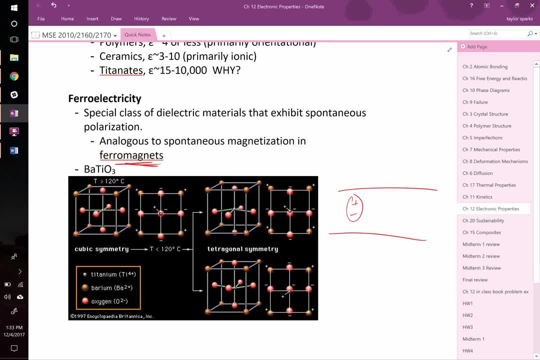 have a Curie temperature above which they lose their magnetization. Basically, all the magnetic moments go from being aligned to being random, And so there's no net magnetic moment. So it started from the word ferromagnet, from that sort of perspective that ferrous materials And then 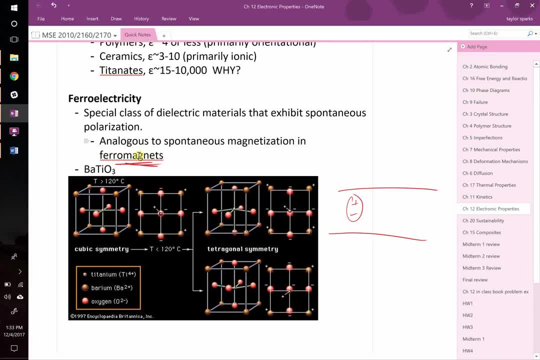 they started observing similar phenomenons, but with other things like electric polarization, And I think the terminology just carried over. It's no longer a ferromagnet, It's a ferroelectric. There's no iron in this. In fact, iron materials aren't like the best dielectrics by any means. I think it's just the terminology. 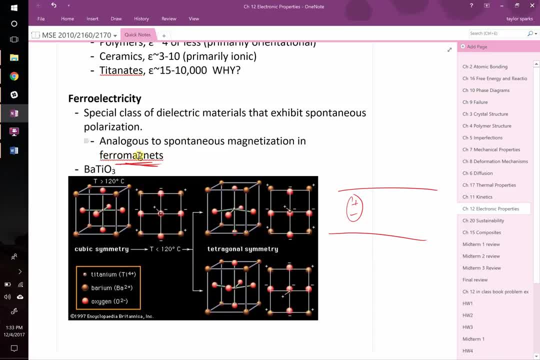 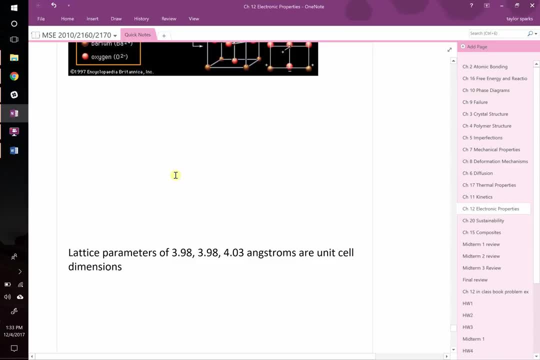 carried over historically. Other questions I can answer. So let's keep going. then We need to introduce something called dipoles, right? So let's say, this is your material, you're looking at under a microscope and you've got a bunch of grains doing their thing, right? 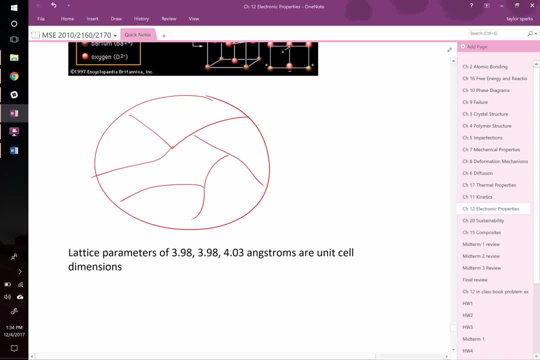 Within each grain you can have something smaller, which is called a dipole. So remember, a month ago we talked about this. We said that there can be regions that have magnetic moments, right, All lined up, And these can be smaller than grains, right You? 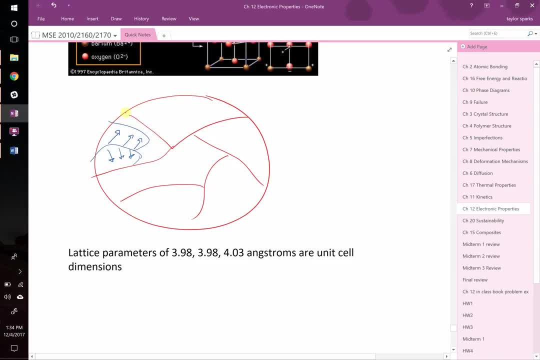 can have, like these little domains which are smaller than grains and they can be randomly oriented, right, Like so. But if you apply a field to these, in the case of magnetic moments, we're talking about applying a magnetic field, right? If you apply a magnetic field H or 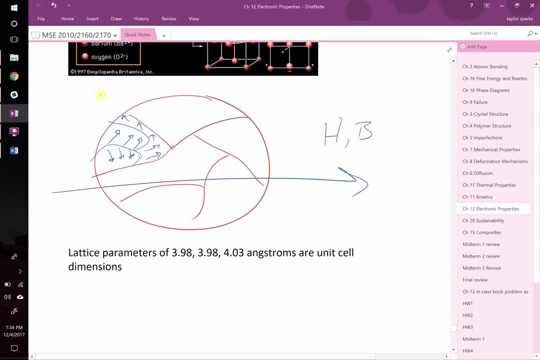 sometimes we'll call it B, right? Then you'll cause these things to line up, right, You'll make them line up, All these different domains, So all these domains will have one net alignment, right? You can do the exact same thing with dielectric polarization. Now you're talking about molecules, right? that are? 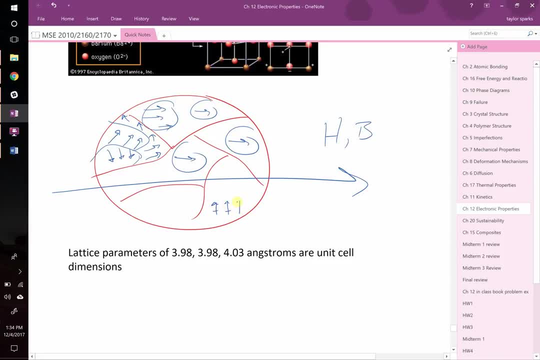 dielectric constants. right, Your dipole moments are lining up like this, right. But again, if you apply an electric field, you can make these things line up. in the same way, All the little tiny domains would line up. If you make them line up, then overall your material is a better dielectric. Any questions? 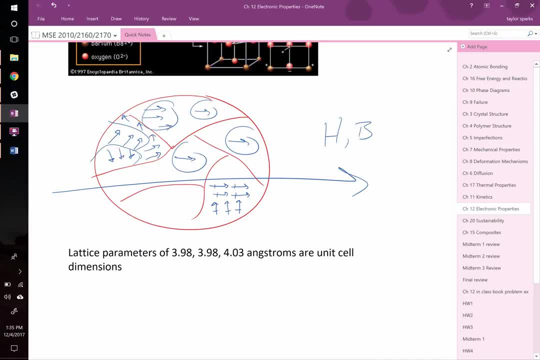 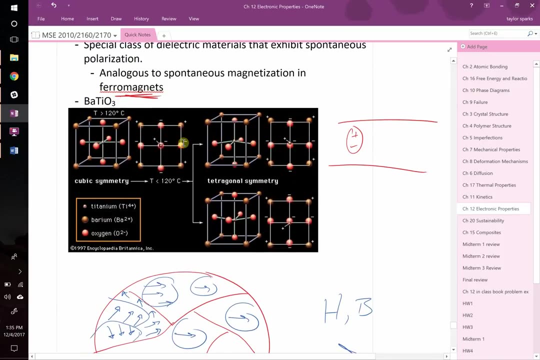 So what next, guys? One way to make them line up really well is to heat it up above its curse temperature, Above its cure temperature. basically, all these moments are just random. They keep on switching. They keep on switching in real-time so that overall, on average, your crystal. 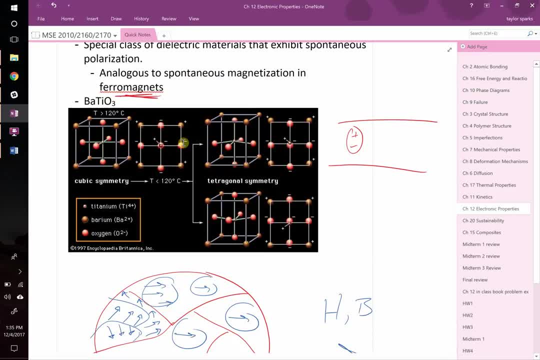 structure looks cubic because the polarization that titanium atoms just keeps on moving all the time And on average its position is centered And so along that temperature it stays above, below a protective layer Right. So the delim chinule on or above the atom is the cholera. 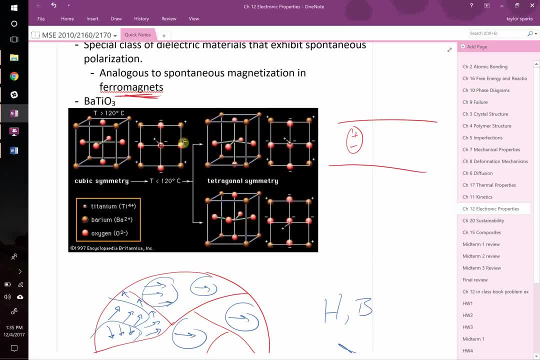 It's making it connect with the earthatra, so there's not enough hippolytes right in it, B producey. It's getting more and more like the cysteine presencephaилach: you can switch it, but it stays put on its own right. so the trick to making really good dielectrics and 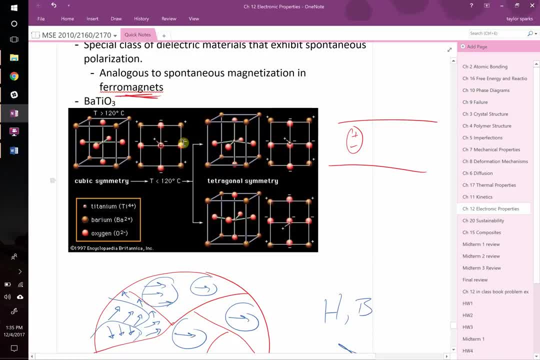 really good magnets is to heat it up above the curie temperature, where all these things are just randomly oriented, right going every which way, and then apply a field which is going to force them all to line up and then to cool it down. so this is called um, oh, it's called polling. it's called 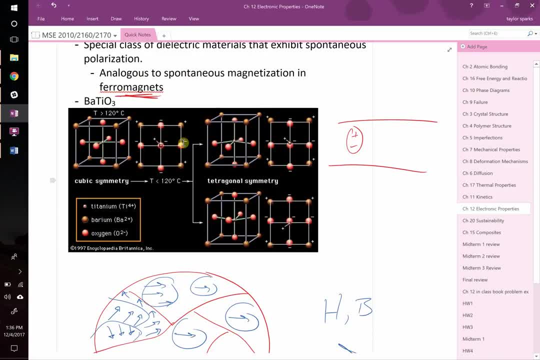 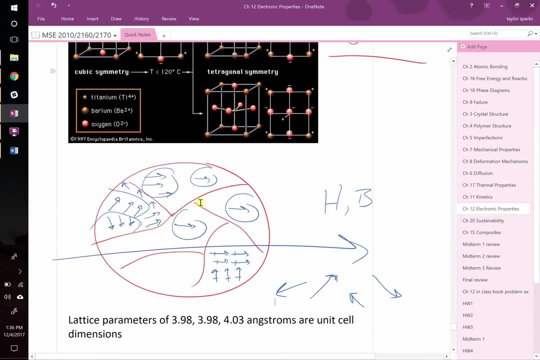 polling. so you heat it up, apply a field- either electric, magnetic, whatever it is the property you're interested in- and then you slowly cool it down and you're going to cause as many of these domains as possible to stay lined up. another way to make a really high: uh, i guess a very good 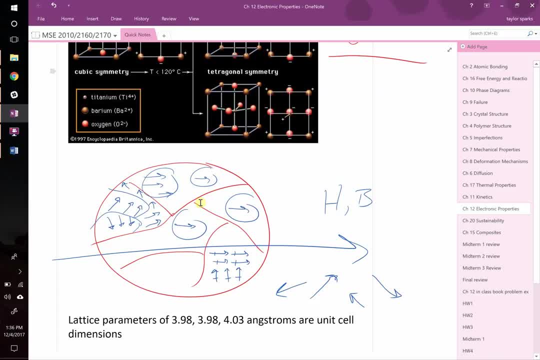 dielectric material or a very good magnet material, would be to grow a single crystal of it, because then you tend to have less of this miscommunication between grains. you get bigger domains, typically in single crystal materials. any questions on polling, on curie temperature, on spontaneous versus not spontaneous: yeah, rosa. 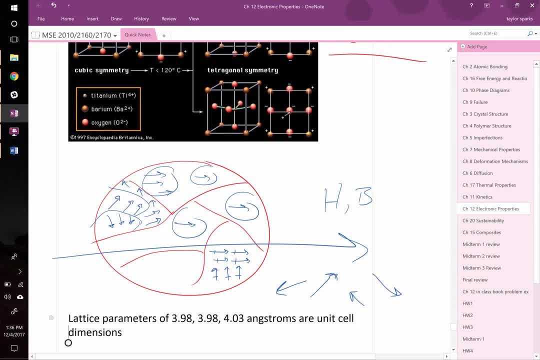 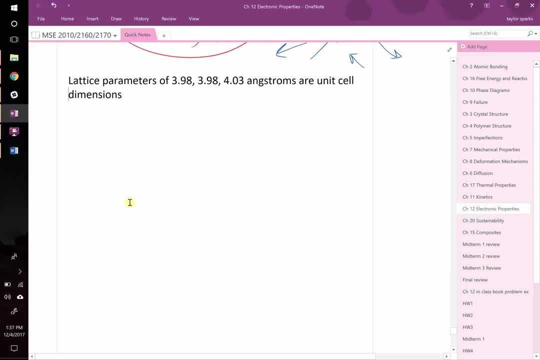 um, so if you grow a single crystal- i lost my mouse. where did my mouse go? there it is. if you grow a single crystal, and it's a true single crystal. let's say you have a tetragonal lattice- right, i'm going to draw it super exaggerated, but every one of these things, 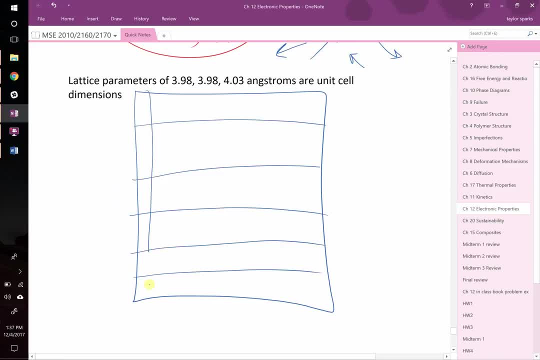 um, they are like taller than they are wide. if it's a true single crystal, then all the way through your material this should hold right. and therefore now, if we start talking about a shift of atoms, let's draw our atoms on here, let's say, like this one's shifted down a little bit. this: 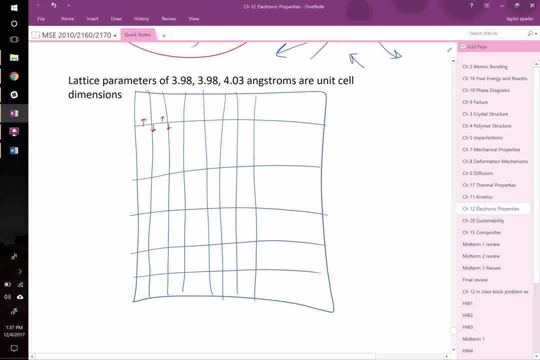 one's shifted up, this one shifted down up, then technically, all the way through, you could have the entire thing, your entire crystal, be one domain which would be switchable right. in practice that's hard to achieve. you get big regions which still are domains, but it's way. 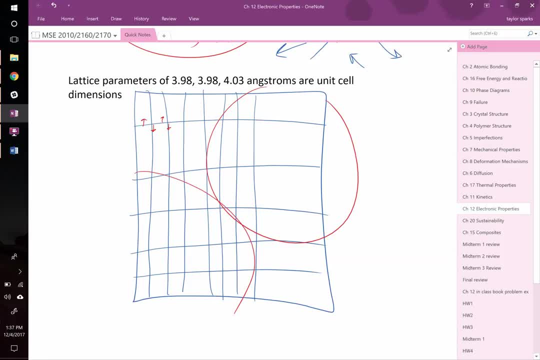 better than a polycrystalline material. Brennan, they do it all the time. that's exactly right. that's yeah. that's sort of the opposite of polling. in polling, you take the material that already existed, you heat it up, apply field to make these things line up whichever way you want them, and then you cool it down, but you 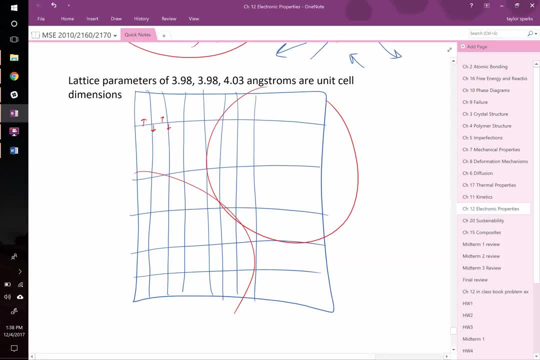 can also grow atoms. so as they attach themselves to the lattice, they do so with preferred spite. so it's called templated grain growth or templated crystal growth. we got Penn State is really good at it. yeah, people definitely do this. they make really good dielectrics, really good magnets by 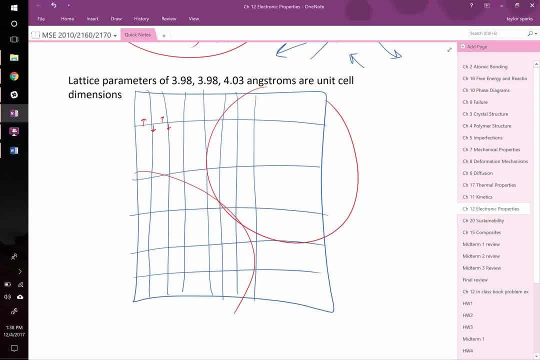 doing this? other questions I can answer about this. I think it's pretty neat, it's pretty cool. it's really cool to go one step further, though. we've talked about magnetic materials, ferromagnets, things that spontaneously, these magnetic moments which are every which way all the sudden just line up on average, right. 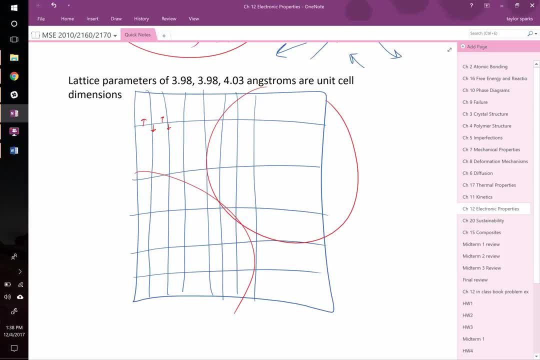 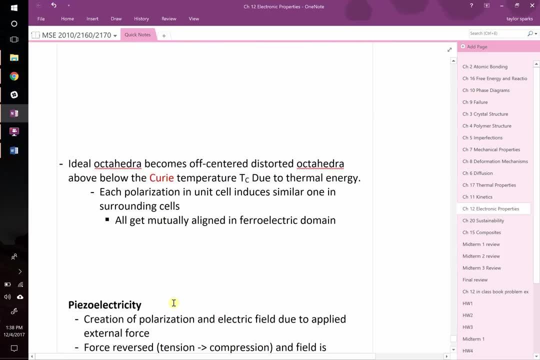 we talked about polarization, where you've got this net positive, negative thing, but they don't work, and they don't work, and they don't work, and they don't, they line up. then you can have coupling between different things. so that's piezoelectrics. let's talk about piezoelectrics. okay, piezoelectricity is. 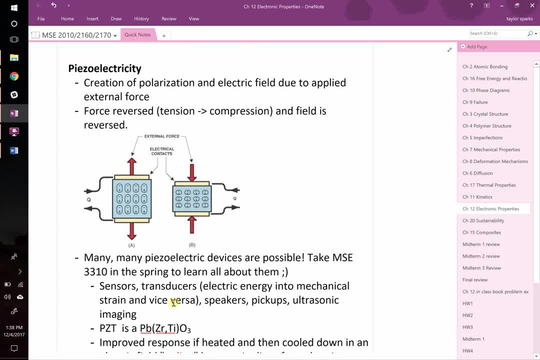 a coupling between an applied strain and an observed electric polarization, or an applied electric field and an observed strain, I guess I just it's an applied stress that creates a strain, right, but it's a coupling between mechanical stress and strain and electrical polarization. so what you can do is you can take this thing. what they're doing is on the 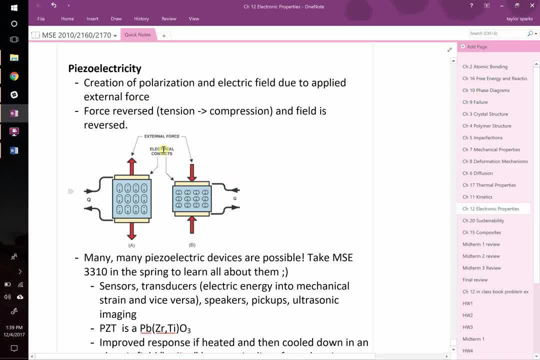 figure on the left, they're applying an external force that's pulling it apart and, for whatever reason, in your crystal structure, when you pull this thing apart, that causes a polarization right of these molecules so you get this accumulation charge on the surfaces, so you actually see a charge occur. and if 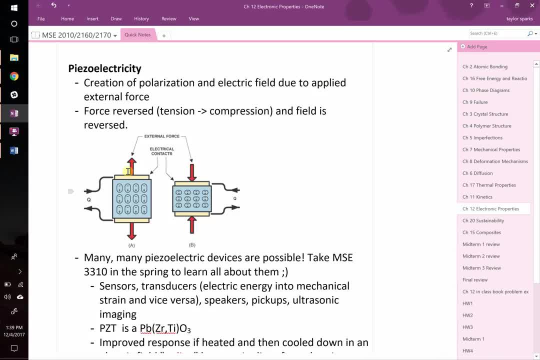 you compress it, you see an opposite charge, right? so these materials, you can imagine, you can make all sorts of clever things with them. right, because you can either create them as mechanical sensors- let's say you wanted it like emission impossible. right, you want to know if the person's like walking on the 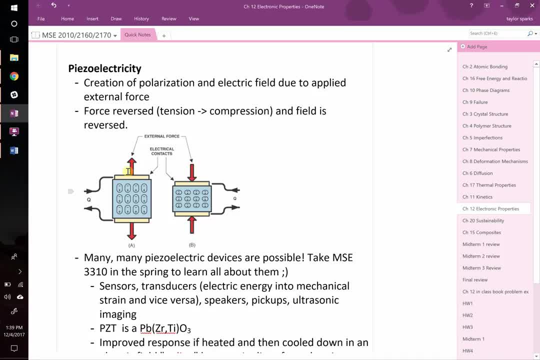 floor to set off an alarm. right, if you step on the floor, it's got a piezoelectric in there. it's gonna produce a small voltage which you could amplify, which you could read in some sort of electrical signal and say there's a pressure there which ought not be there. right, you can make pressure gauges like 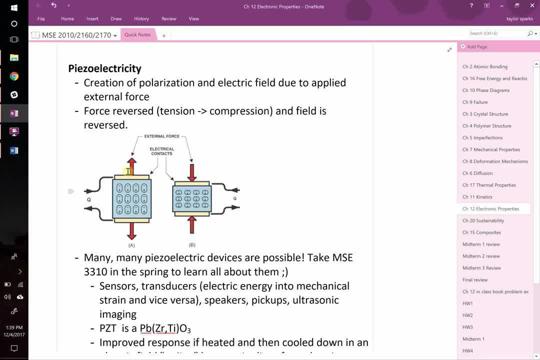 that in our group we do that all the time. we actually make these underground so in the dirt, make tiny, inexpensive sensors for detecting moisture. how they work is: we take a polymer that can swell in the presence of water, We butt it up against a piezoelectric sensor. We have these things swell with water, which causes a swelling pressure on. 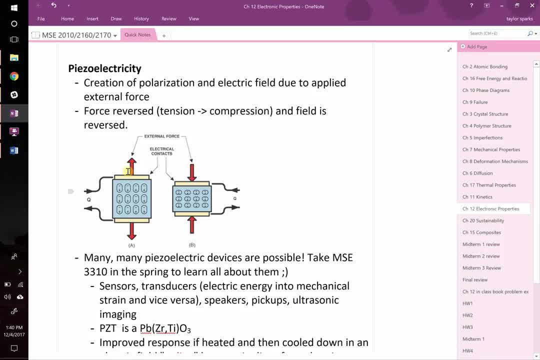 the sensor And we can back calculate what the soil moisture should have been right In a cheap and easy way. I say we, but I don't do very much. It's mostly Dr Bates in my department. right, You can do this for all sorts of things. You could go the other way. You could apply a voltage. 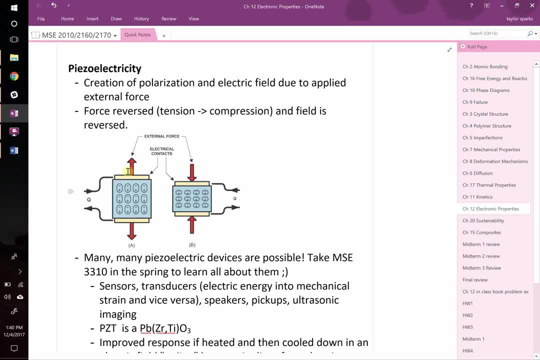 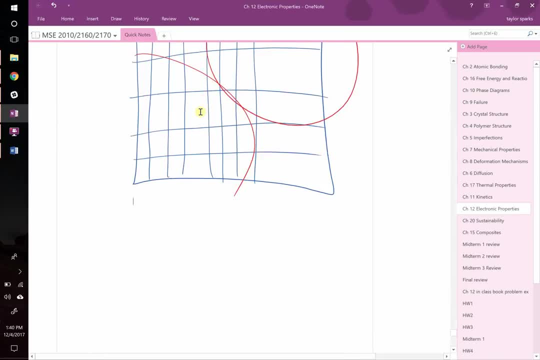 and cause these things to collapse or expand a little bit. Now, on an individual unit cell, you're not talking about big changes, right? If you go back to our barium titanate, I had showed some lattice parameters. Instead of being perfectly cubic, 3.98 in all three. 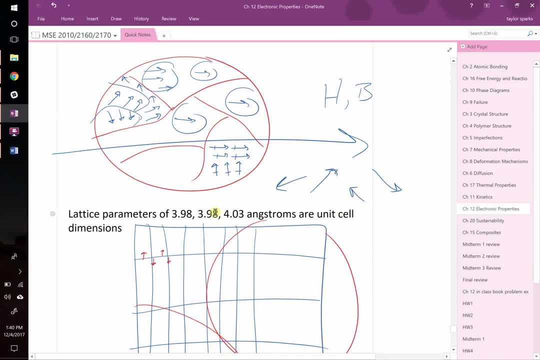 directions. this one, its polarization goes from 3.98 and in one direction it goes to 4.03.. So it's like fractions, like a percent or two. right, It's very, very small changes you're talking about, but sometimes you don't need big changes. In fact, we use these for fine motor control. 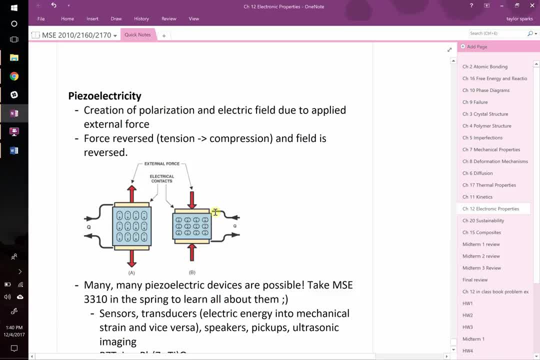 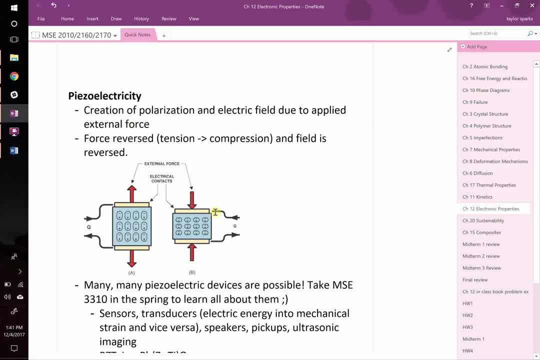 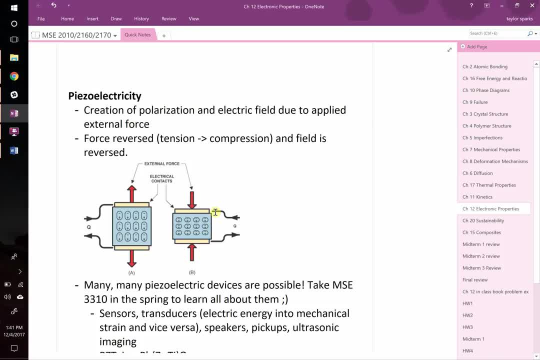 like poke, that with your finger You're going to send it like miles too far, like relatively speaking, right? So instead, what you do is you have a tiny little piezoelectric which can shift things really small amounts at a time. right, We use these as vibrators, right? If you, instead of 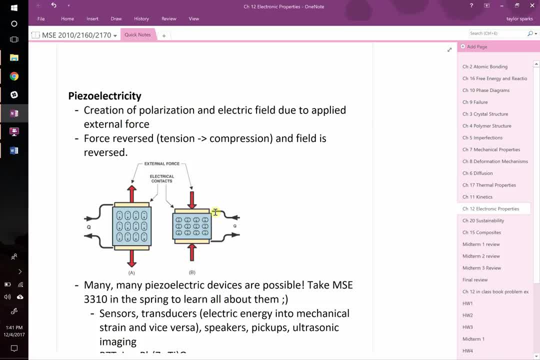 having a constant signal, right, A constant DC, direct current. but what if you alternate that? Now you're making the atoms shift back and forth. right, you can actually produce a strain that vibrates back and forth. So buzzers and phones, all sorts of things, you can make those out of piezo electrics. 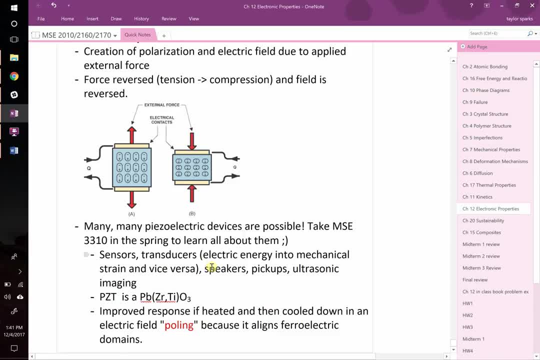 sonar transducers. If you ever had looked at a baby under ultrasound, all of these things take advantage of piezoelectricity. in ultrasound You basically take a transducer, something that vibrates. it sends now a pressure wave into the belly right. That then bounces off the forehead of your kid and bounces back to another. 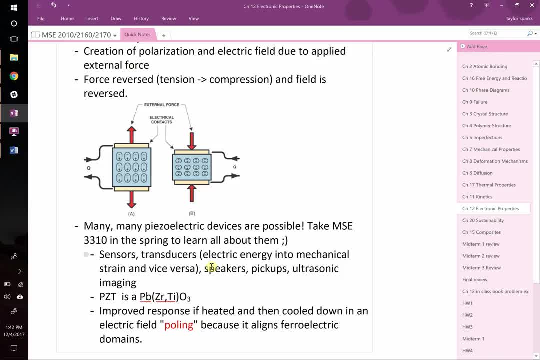 Transducer that picks up that signal and from the time distance it calculates a 3d image, right, Which is pretty darn magical. Yes, me right, You can find submarines, you can map the ocean floor, You can find fish like these things are everywhere now, like all over the place, and they're pretty amazing. 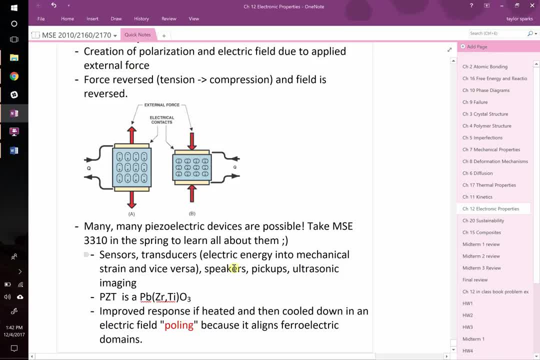 This is how speakers, pickups, ultrasonic imaging, all these things work, because of this clever principle That if you apply a strain, you observe a voltage, or if you apply voltage you apply a strain, you get a strain out of it. Right, That's piezoelectricity. This gives rise to a whole new family. 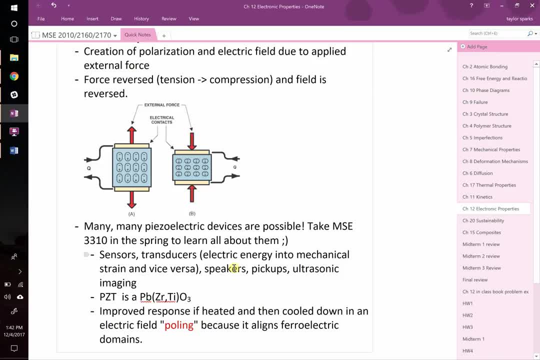 Materials which we call multi ferroics. So again going back to the whole ferro, ferro magnet for electric Multi-ferroics are things that couple one or well two or more Ferro things that can be magnets. There's things called ferro elastics. There's ferro magnets for electors. 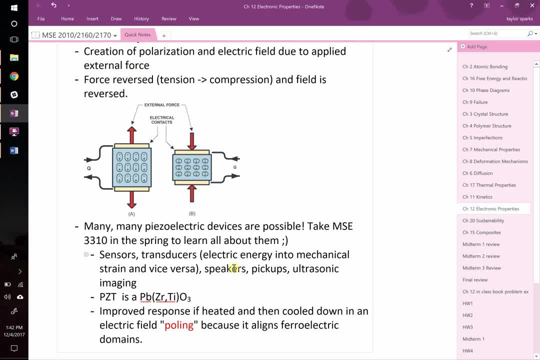 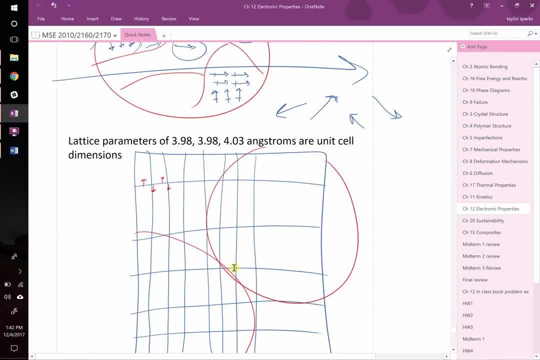 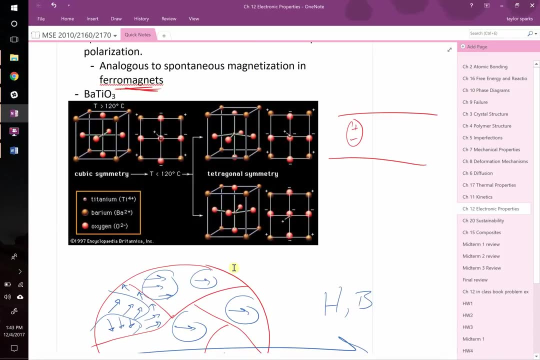 We won't get into the details in this class, just realize that they exist, that you can couple them in principle, but in practice It's hard. It's hard to find one magical crystal structure right, something like Like this that just works for Everything, that basically you could take an applied magnetic field and get a polarization right- electric polarization. 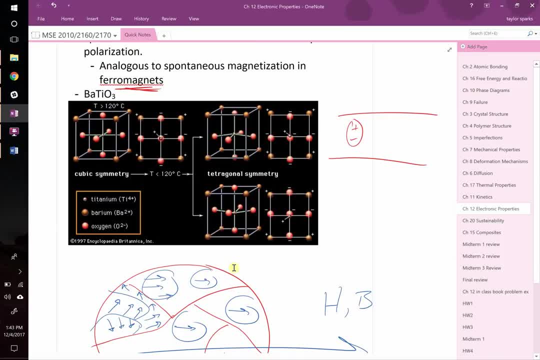 That's hard to find a material that does that. it's easy to find a material that you apply a strain and you produce a polarization. So what they do instead when they want to get these interesting cross Field couplings, what they normally do is they they rely on second-order coupling. Here's how they do it. It's pretty clever. 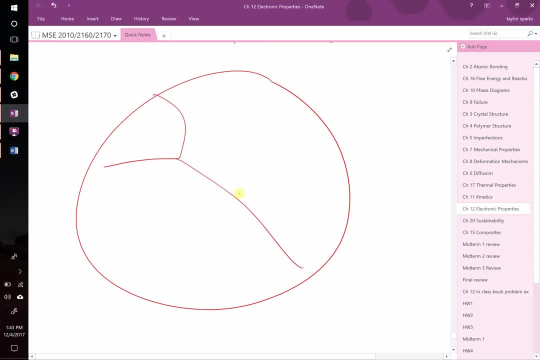 So let's say you've got your material here and you've got two different types of materials in your overall material. So it's a composite right. You've got like material a and you've got material B. So let's say that material a is a ferroelectric, piezoelectric, so piezoelectric.